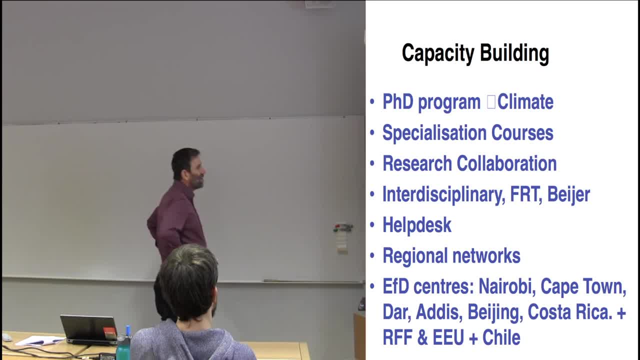 We do quite a lot of research. We have a collaboration that is sort of interdisciplinary and there's, I think, two or three of you here from physical resource theory And that's one group we've worked a lot with at Chalmers. 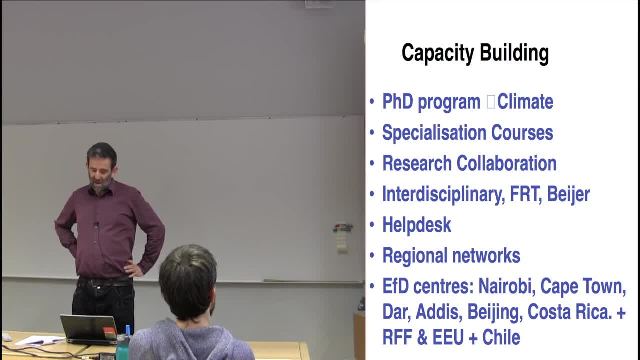 And now we're working quite a lot with the Bayer Institute- and some of you were there a few weeks ago- And we have started these centers that some of you know about, called the Environment for Development, And we have a number of development centers in a number of places which we collaborate with. 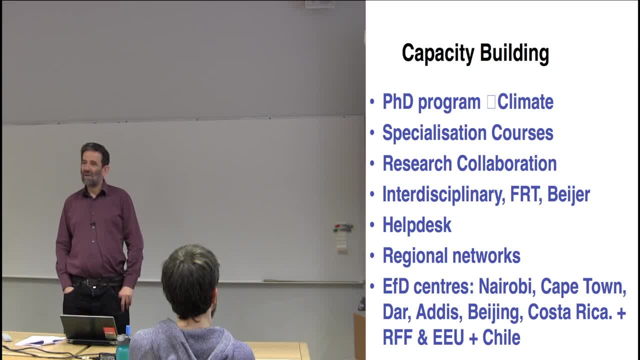 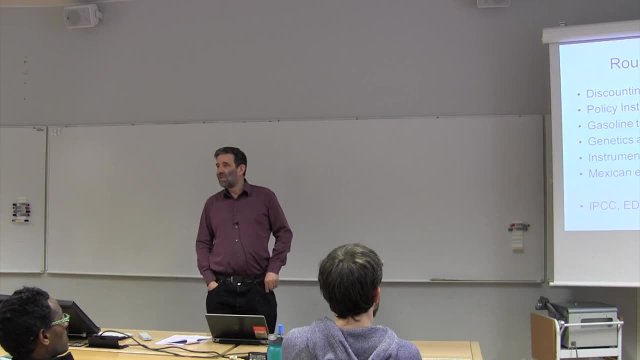 And we're now all writing a gigantic research application, together with the Bayer and the Stockholm Resilience Center and all these centers, and planning for more money to do research the next 10 years. I thought we'd do a little quick round of presentations. 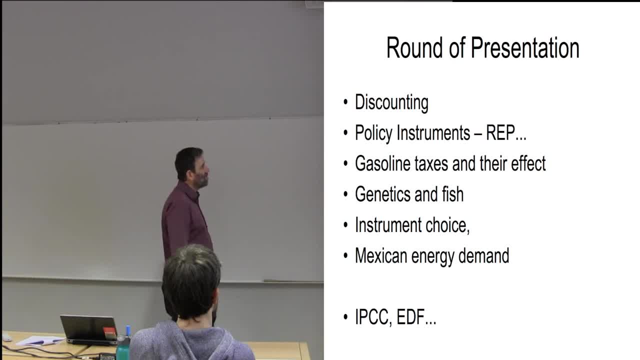 so I wrote down some of my own personal experiences. I've been working on the policy of interest, I've been working on discounting- And I'm going to put in an extra lecture into this schedule somewhere- I haven't quite decided yet where- on discounting, 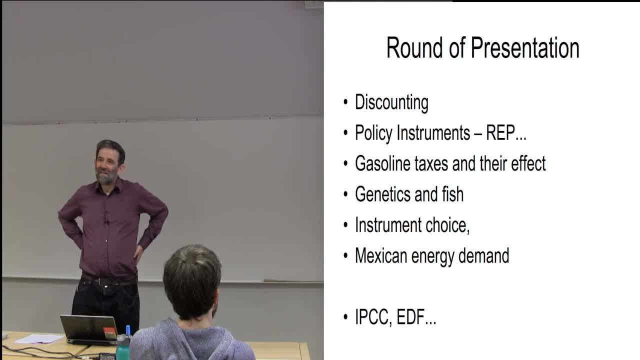 We were going to have one in the Natural Resource course, but then I got ill And so I thought I'd squeeze that in here. It fits just as well. It's sometimes been in the Policy Instruments course and sometimes in the Natural Resource course. 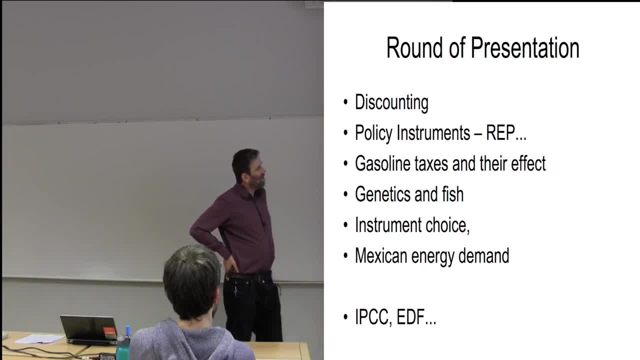 It fits in both. I've also worked on the design of policy instruments, And particularly one for the refunded emission payment, which we'll talk a bit more about. I'll have a lecture next week on that. with Carolyn Fisher, I did a lot of work on gasoline taxes, my favorite policy instrument. 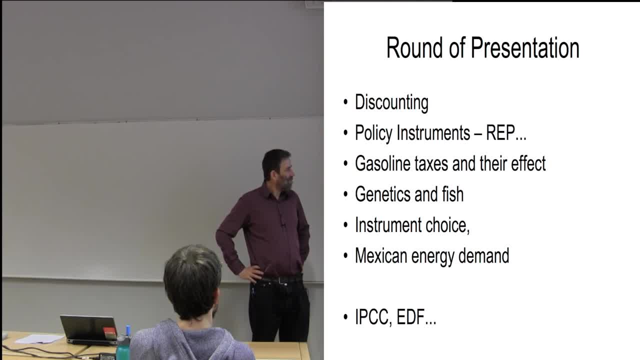 And a number of other things. I wrote my thesis about Mexico And currently I'm involved in the IPCC. I'll be gone ten days of this course. I'll be locked up in Berlin. I'm not allowed to leave. It seems it's 24 hours a day. 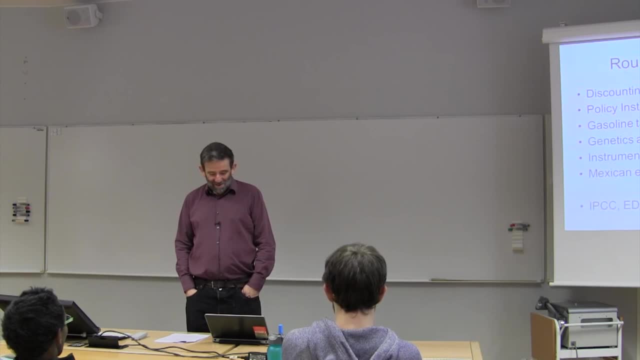 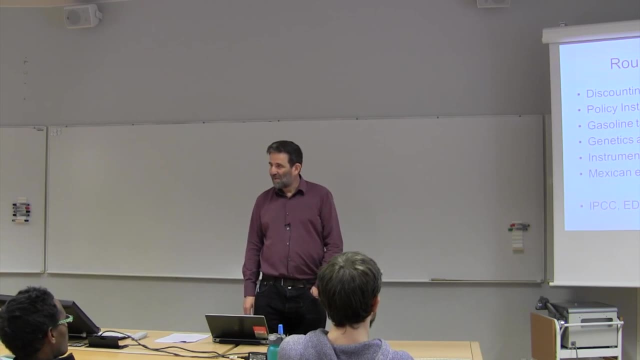 So I'll probably come back a little tired and quite frustrated, I'm afraid. And then I'm still working also for the Environmental Defense Fund, which is a sort of an advocacy organization in the United States. Now can we do a little round-up with this? 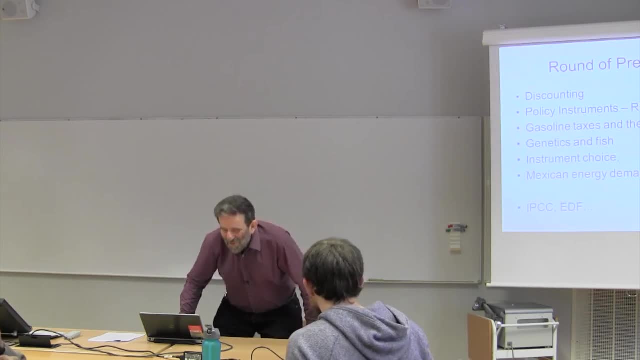 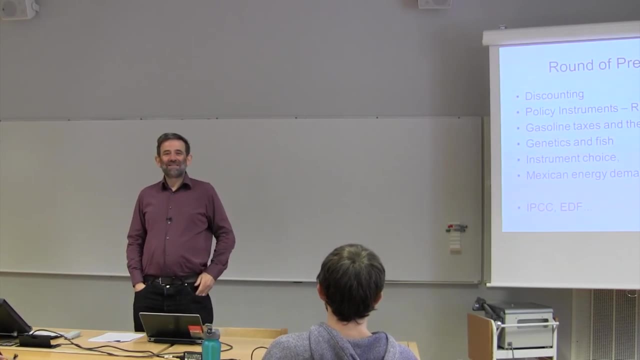 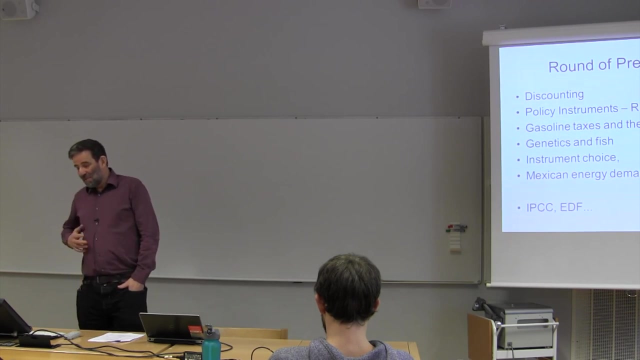 There's some new people. We have a wonderful span of people from these outer space cloud researchers here to people looking at common property, resource management and grazing and many things in between, like urban problems in China, And that has been. it's been a privilege and a joy to have this as my area of specialization. 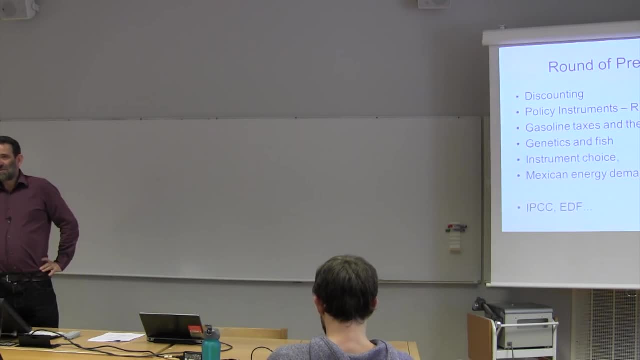 I say that with some kind of- you know- citation marks. We always tell economic professors, always tell their students, and I suppose probably a lot of other professors too, that you must specialize on one thing, And so I specialize on policy instruments. 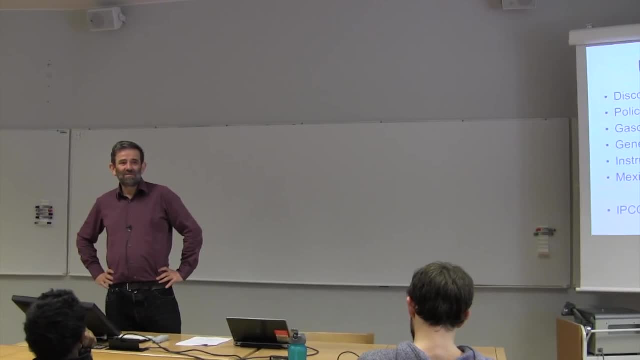 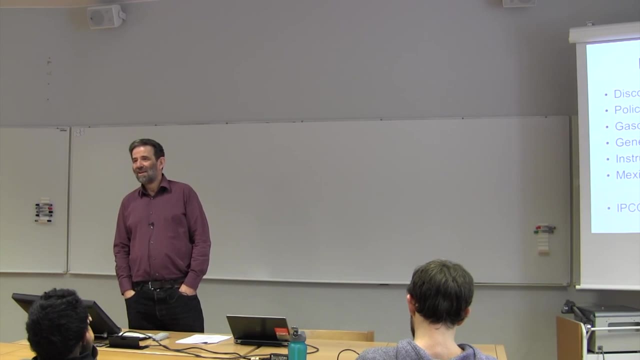 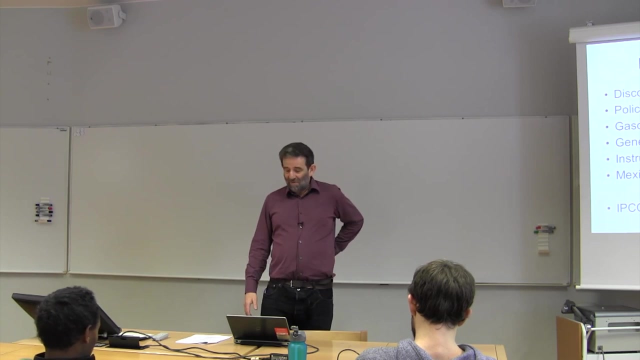 And it allows me to work with all these different subjects, And sometimes there are really striking similarities: We use the same policy instrument to manage fisheries as climate forces like carbon dioxide, So it's quite interesting: We actually collect experiences from one area and use it in really very different areas. 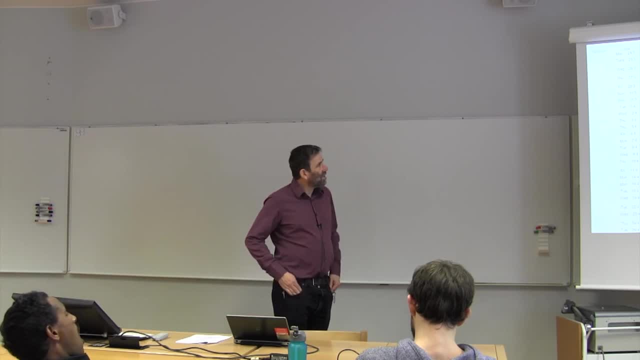 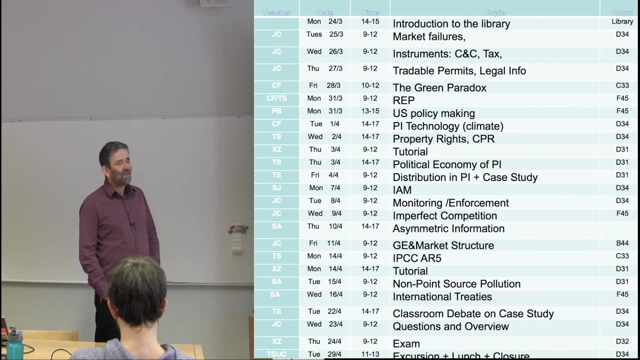 So this is our schedule. Those of you who are new- if you are new to the school here- we'll have a little introduction in the afternoon about the library and the school and so on. Then there'll be a block of lectures this week. 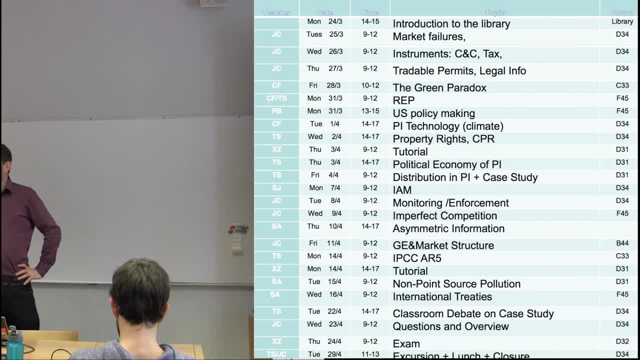 Market failures, which is sort of the reason why we have pollution and environmental degradation. Then we'll have a couple of lectures on what, what policy instruments there are to deal with this. Caroline Fisher will come and give a lecture on the green paradox here. 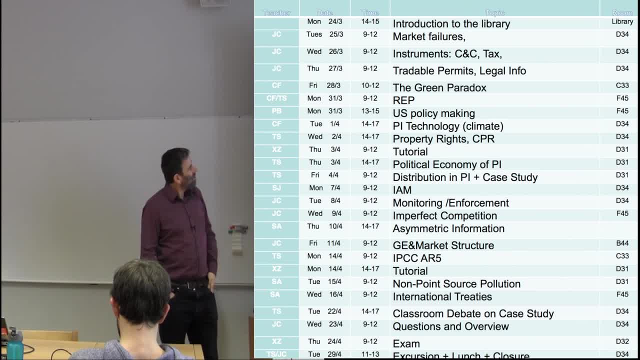 And she and I will together give a lecture on refunded emission payments. Peter Burke will give a lecture on US policy making in practice. I'll come back here with one on policy instruments and political economy of policy instruments. There'll be a case study. 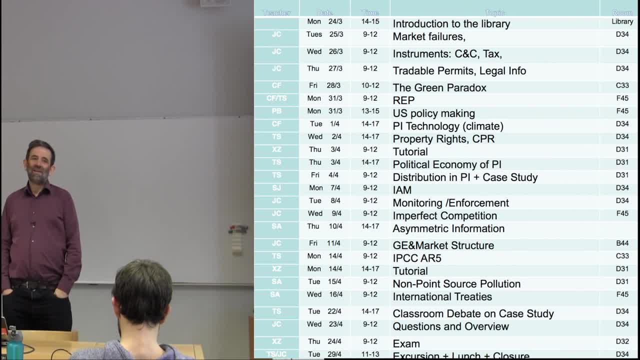 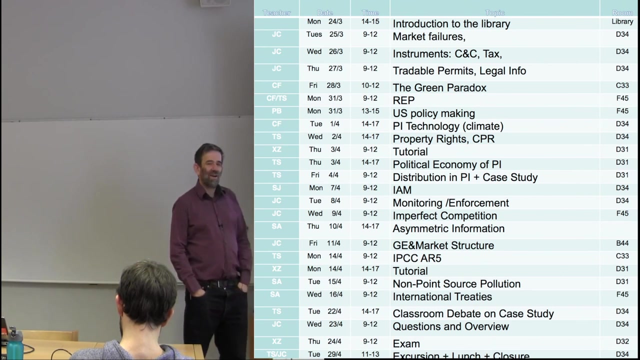 So you will be. this is a so-called Harvard case study. You will be divided up into little groups and you'll have one company each and work out a lobbying strategy to try to find which instrument is best for your company. And well, there'll be a lecture on integrated assessment modelling. 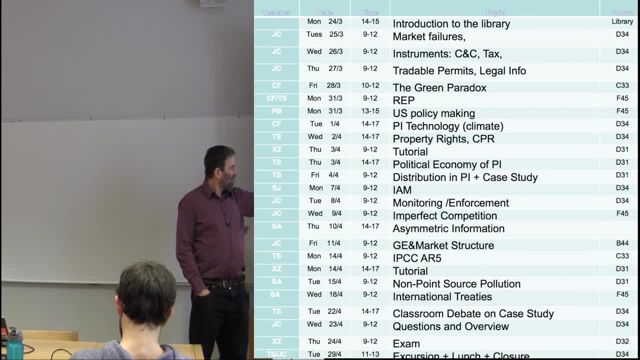 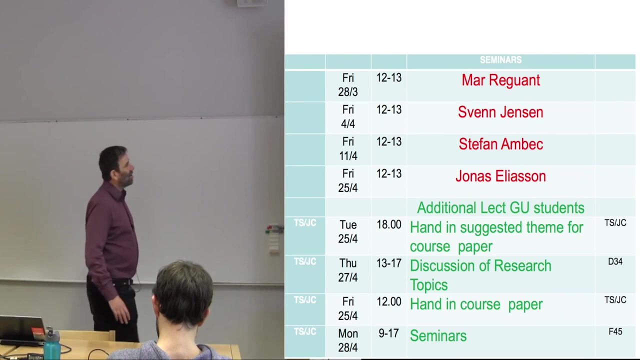 some on monitoring and enforcement and so on. I'll give one on the IPCC fifth assessment report, which will be just after it becomes public, International treaties and so forth. There's a little bit more Here. there are the four seminars in red. 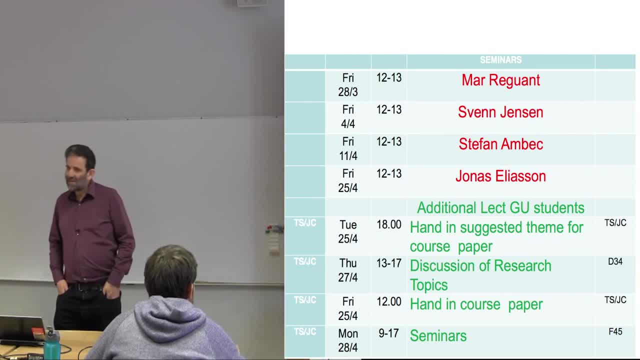 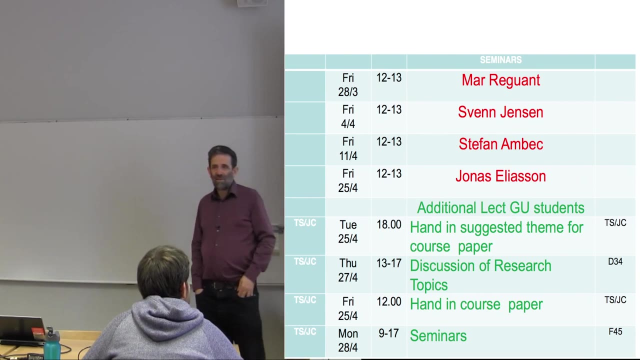 They are in your schedule. They are seminars and they are designed to be specifically about the related topics, So they are very strongly recommended. And then there is three or four things here that are specific, just for the PhD students that are our regular PhD students here in Gothenburg. 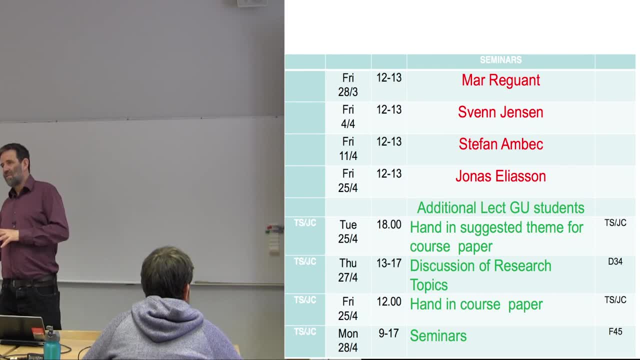 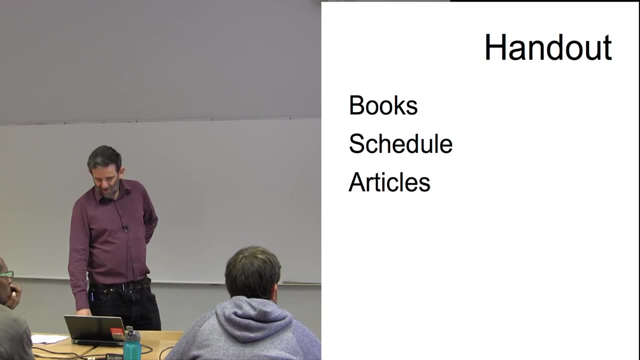 They will be writing a term paper that is also associated with another course and to this one, and so that's a little bit specific for them. I'm going to hand out the books afterwards. The schedule was handed out and the articles we don't hand out because that's illegal. 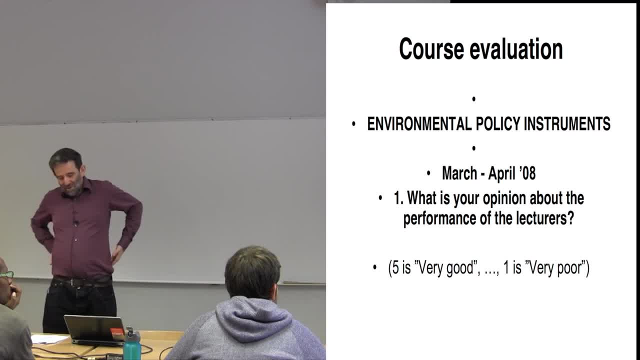 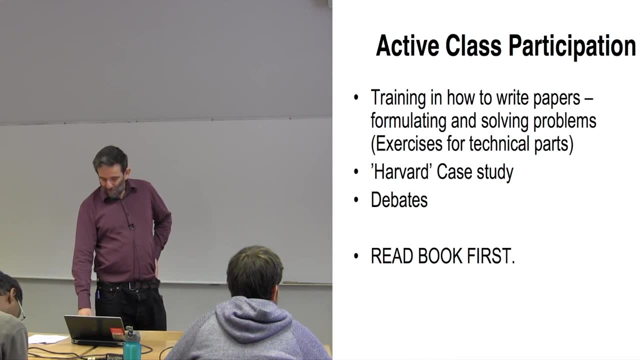 At the end there will be a course evaluation. We do this at the end of every course. We ask you lots of detailed questions about what you thought about each lecture and each thing, And we use that as feedback to make the courses better. of course, 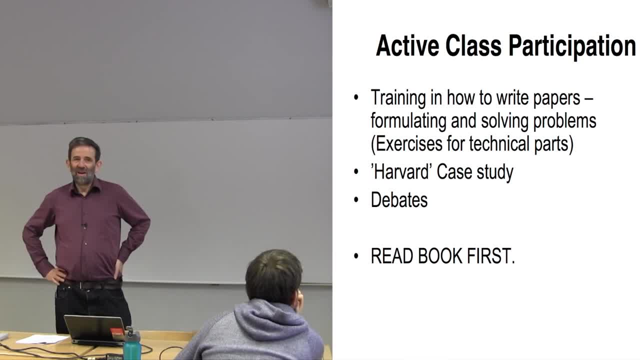 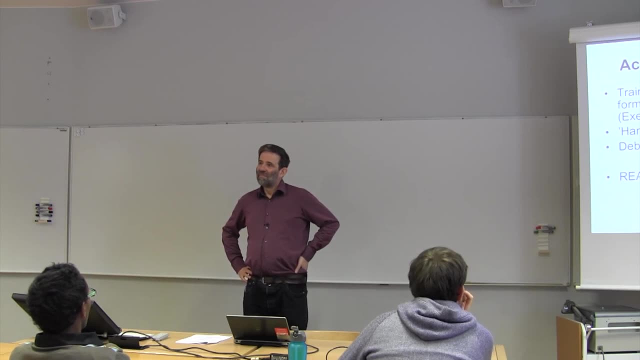 We'd like you to read the book as soon as possible and sort of have that as a basis for really participating. It's a big group but still We want to get active Participation. The purpose is for most of you is to think about your thesis. 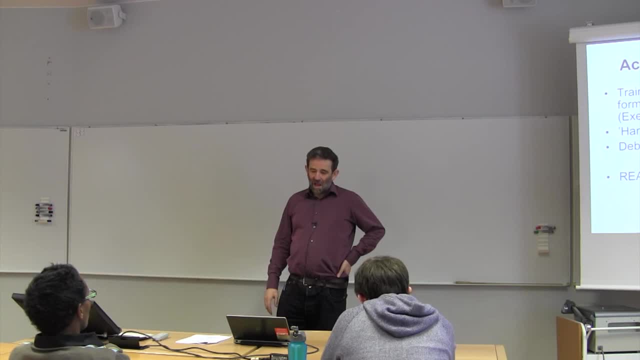 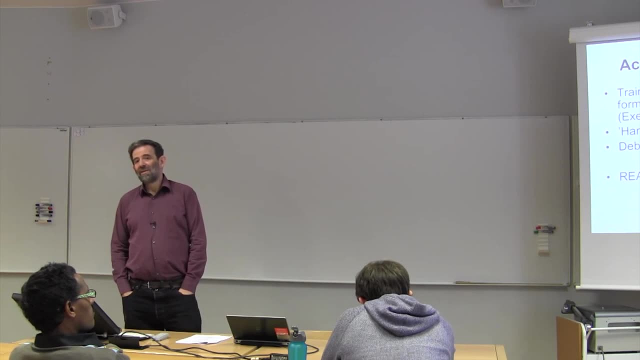 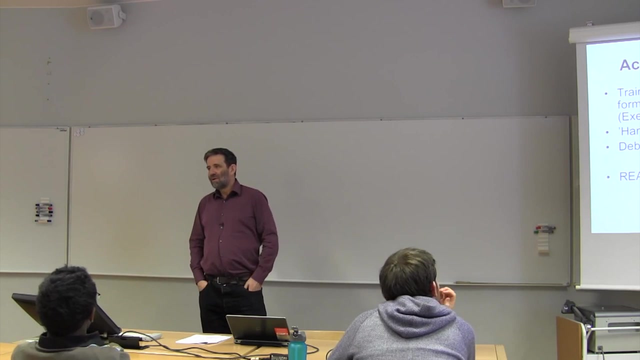 Most of you are in that stage where you will soon be writing a thesis, And this course, I think, is well designed for that kind of purpose. So you might be thinking about topics that are specifically oriented to the design of policy instruments, Or you might also even if you are not and you're writing a thesis about something else. 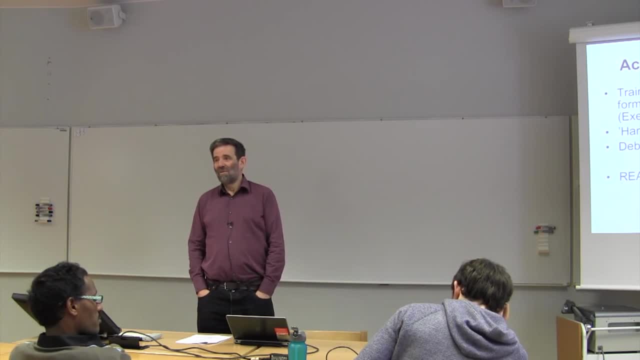 there is very often at the end of every thesis, chapter and article there is a page or two where you kind of sum up why you did this and what the consequences are, And that's the time to think about this course And this literature. 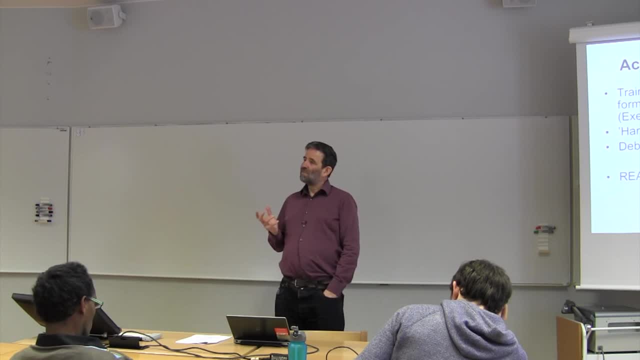 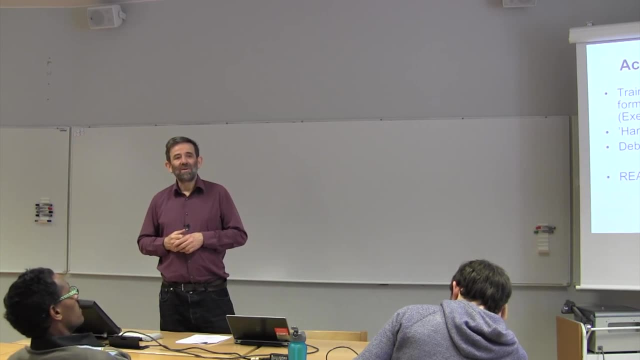 Because it makes a big difference if you kind of can explain: You valued something. Very many studies value the local lake or something and try to say something about what it's worth. But then you need to like, as a conclusion, to say: 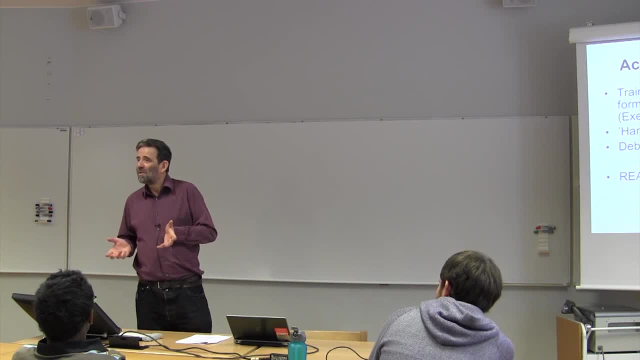 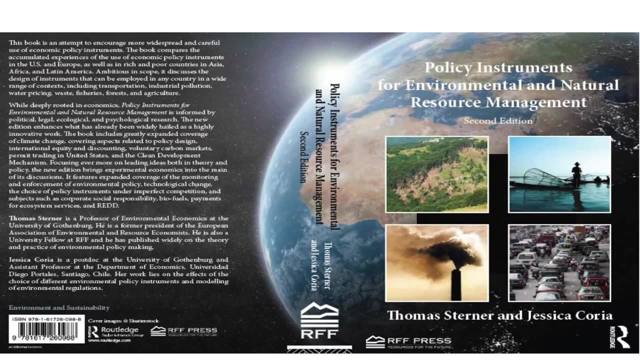 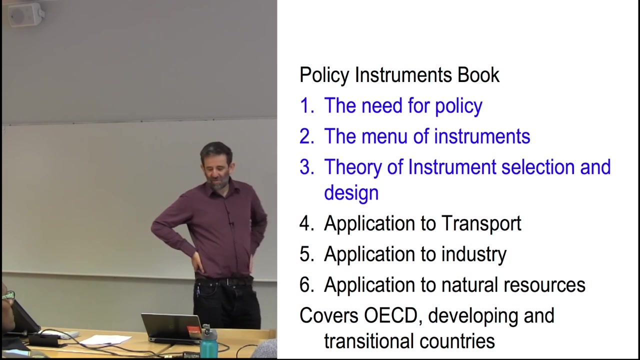 well, what's the conclusion of this? So what should the policymaker do? And I think that's very important. This is a book, And the book has six parts, And we'll be talking today a little bit about the first three, and then the other three are applications. 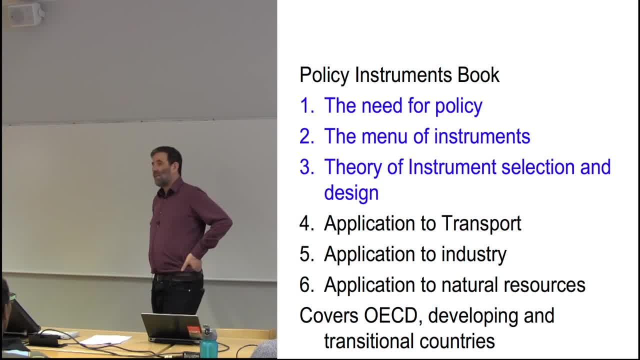 But there are three different parts And I think you should always think about this when you think about a new problem. Why is there a problem? Why do we need policy? Some people think this is sort of obvious: That there is pollution and that there are problems. 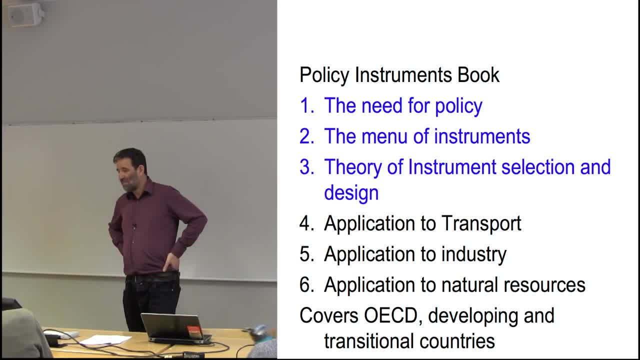 But it's not obvious. Particularly not obvious perhaps to people who've had a long training in economics, because we are taught that the market economy is so great and sort of the best way of allocating resources. So then we have to ask ourselves why, if we have a market economy, 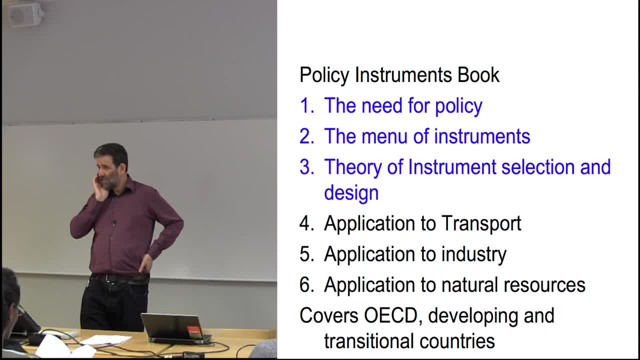 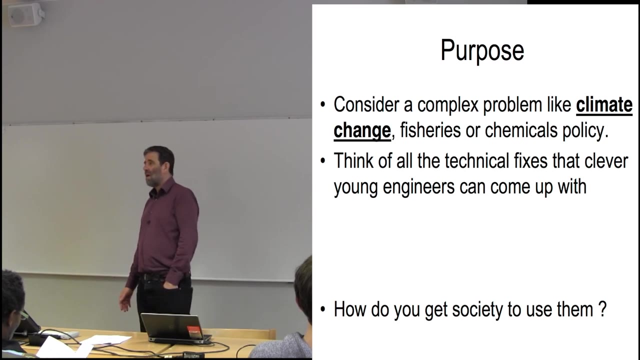 then why do we still have these rather serious problems? And then we want to look at the menu of instruments, what there is to do about this, And then the really big subject is which instrument you select when So think of a complex problem. 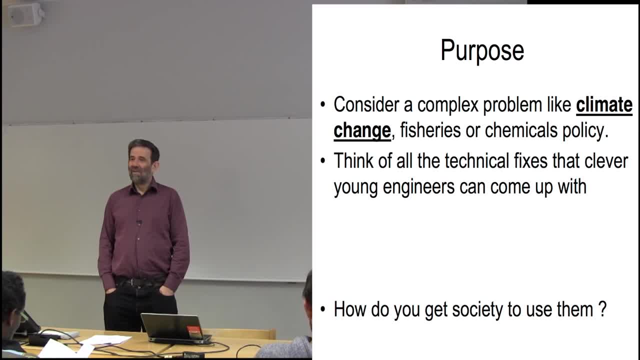 And we have some people here from engineering school. They are very good at figuring out new ways of making lamps so that they use less energy, or pumps so that they use less energy, or all kinds of technical innovations. But then how do we actually get society to use this stuff? 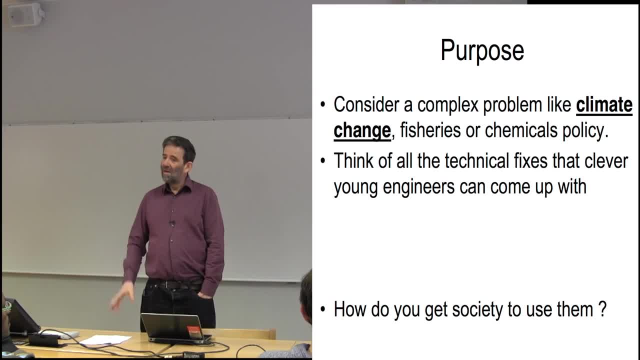 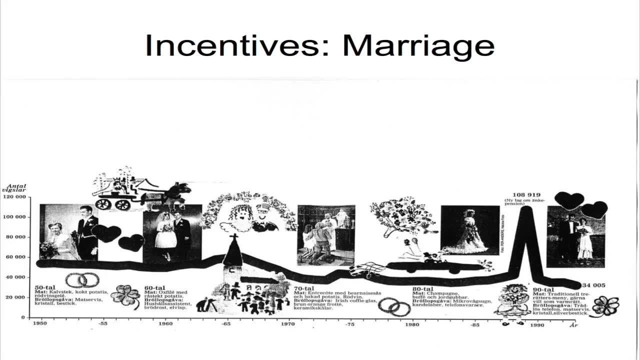 And how should society be steering research? And I'll take as an example here of the importance of incentives A diagram which was taken from a daily newspaper in Sweden called Dagens Nyheter. It shows the number of marriages in Sweden. In 1950 there were almost 60,000 marriages a year. 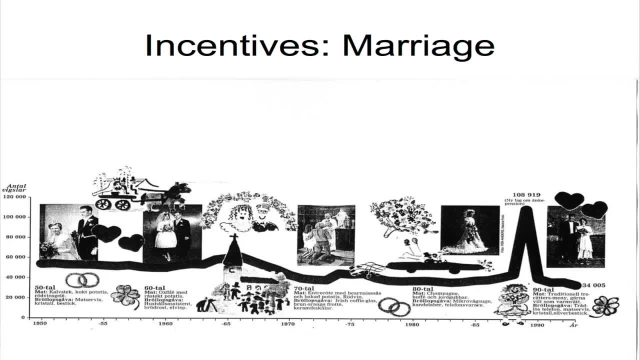 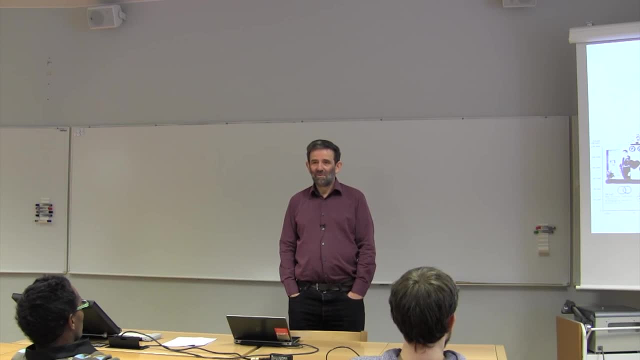 And then it fell. I think the lowest was about 1980 here, when it was down to about 35,000.. Do you know why it fell? Less people, people already got married, nobody left. What explanations would there be? 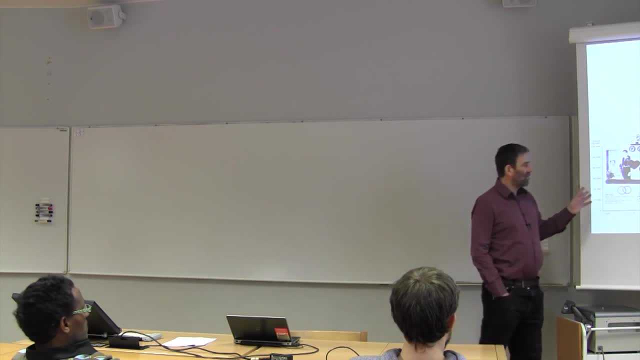 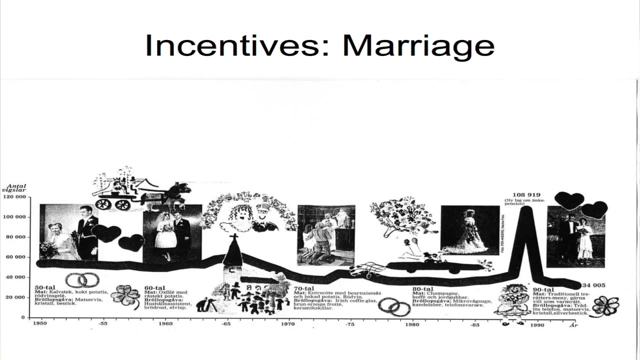 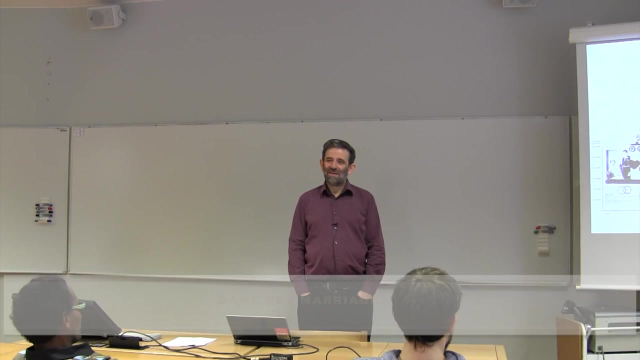 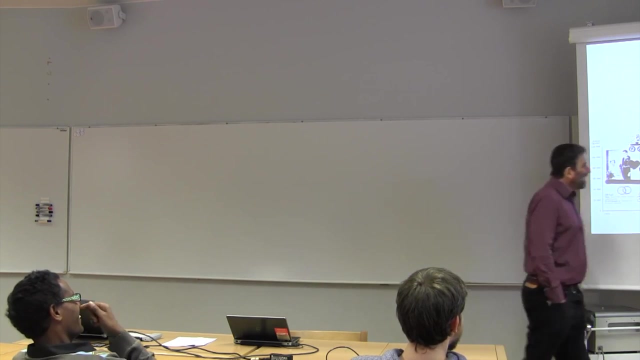 It was the power- largely the power of the church was getting lesser in Sweden. And then there was one year here in 1989, when suddenly 109,000 people got married. I think that came a little bit later actually, so I don't know. 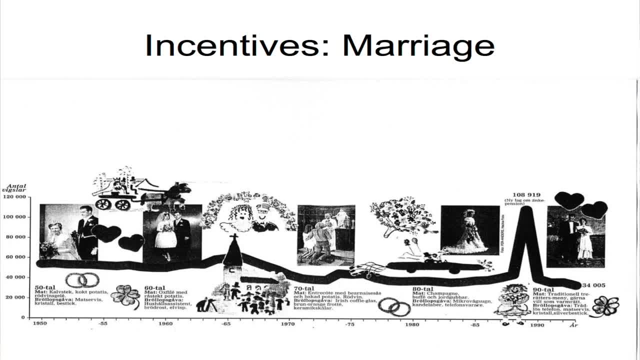 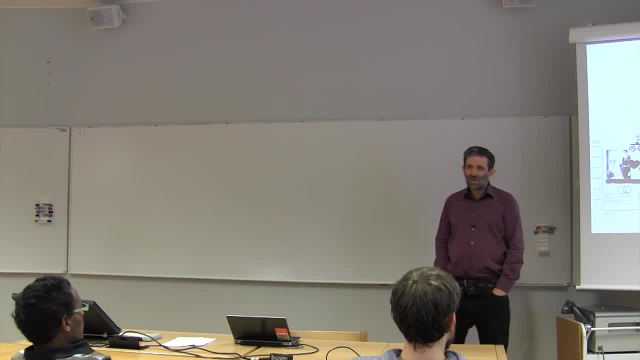 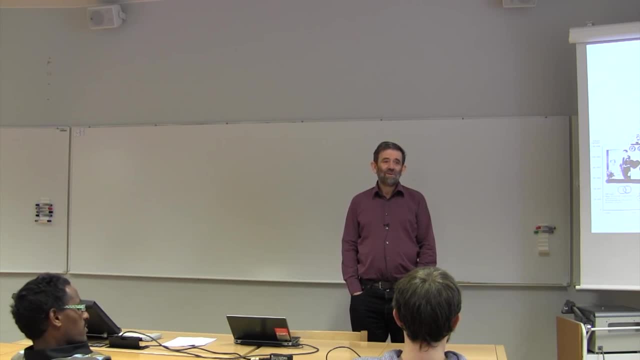 Maybe I'll have to update this and see if there was a new peak, But actually I don't think that had such a numerical effect. No, there was a change in the law about how widows' pensions were calculated, So it somehow became just more profitable to be married. 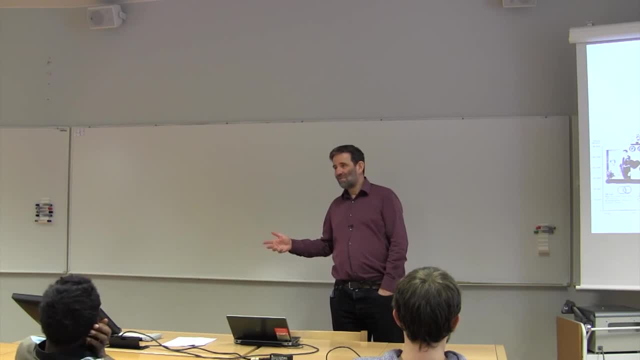 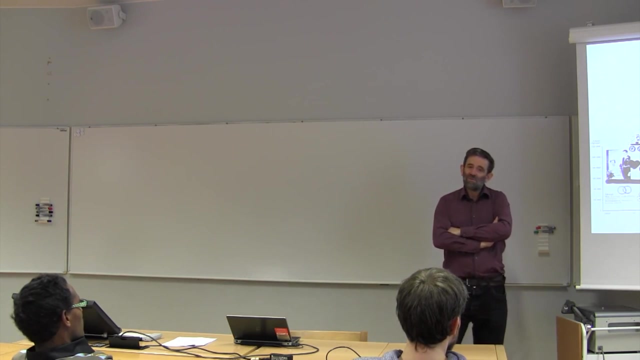 There was an opportunity cost of living together and not being married, And if one person died, something about the way the other person's widow benefits were calculated or taxed or something. A seemingly small sort of financial incentive has such a big effect on something so personal as marriages. 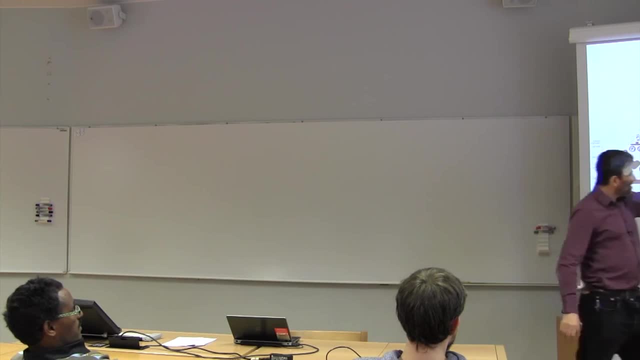 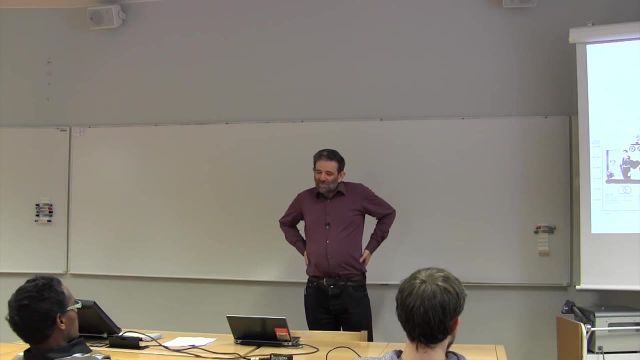 Then it goes back again. yeah, But still I went to the same level, so there's still a lot of extra people who got married there. So I show this diagram because I've been fighting for decades to persuade people that gasoline taxes have an effect. 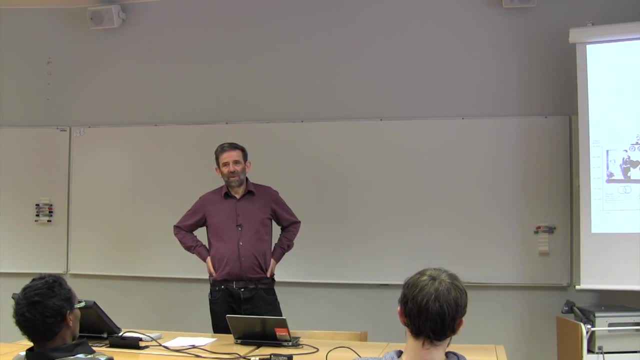 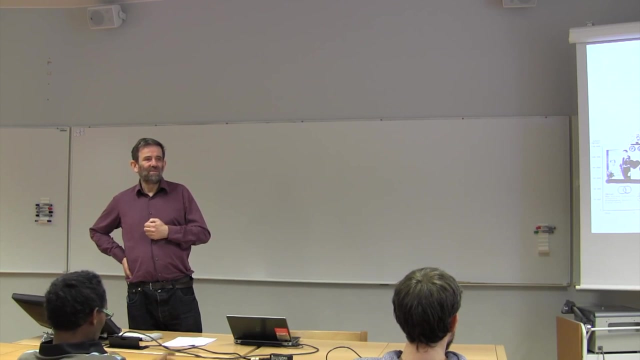 And I looked for different ways, because there's always some people who think that they don't. Those people are wrong because there's lots of statistical evidence that they do have an effect, But still they continue to believe that there's no point in taxing gasoline. 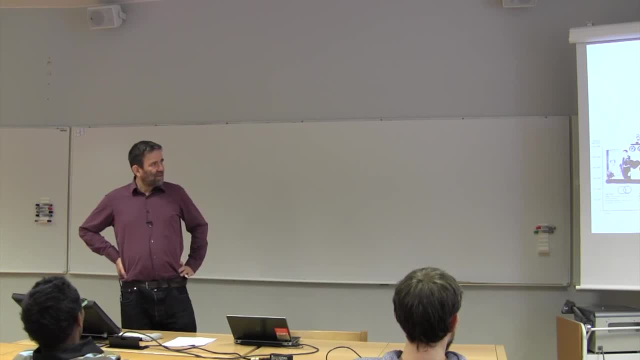 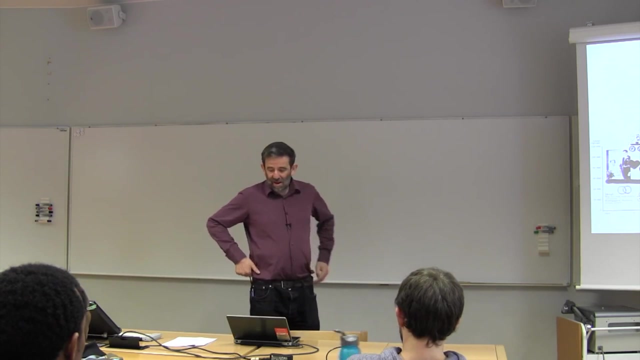 So this is to show that if an economic incentive can have such an effect on when you get married or if you get married, then it can surely affect lots of other things like what size apartment you choose or what kind of car you choose. And people sometimes say that 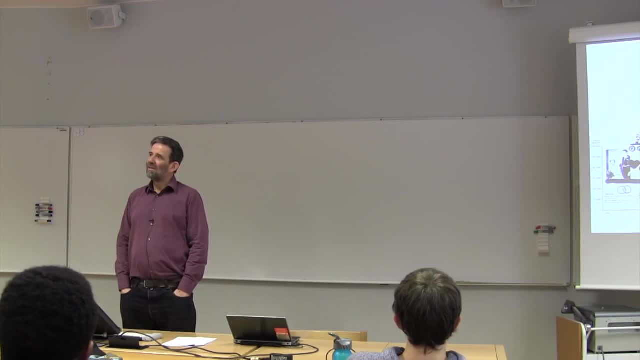 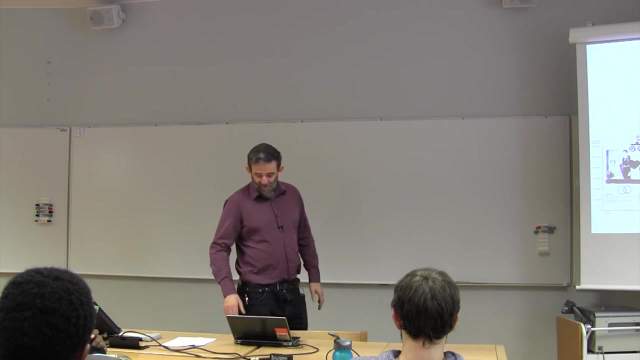 you know it's all a matter of culture and so on, But many things, like culture, as well as technology and so on, are ultimately decided by prices. Prices are really important in a market economy, And so that's the most powerful instrument we have. 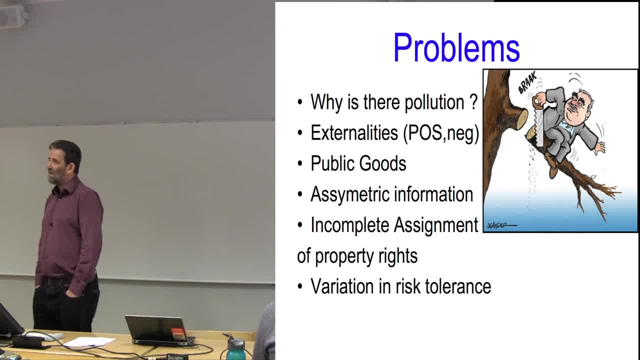 Now let's come back to the question of why we have environmental pollution. It's really stupid to destroy the ozone layer, for instance, or to change the composition of the atmosphere so that the climate on Earth will change. Why do we do it? 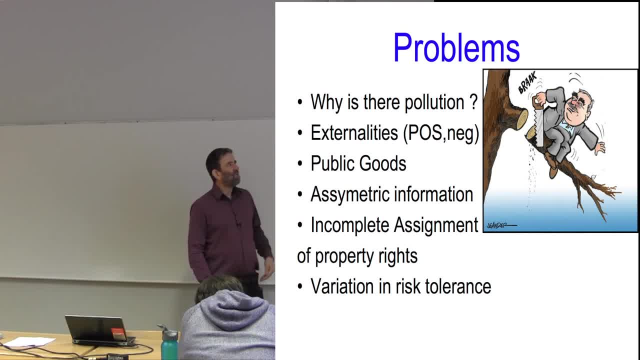 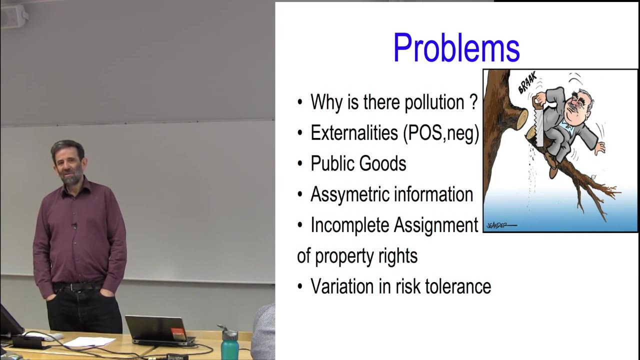 It's important to think quite a long time about this, because there's a risk that if you have a superficial understanding of the problem, you come up with a superficial policy recommendation And there is generally a fundamental reason. The market does work very well, if the market is allowed to work perfectly. 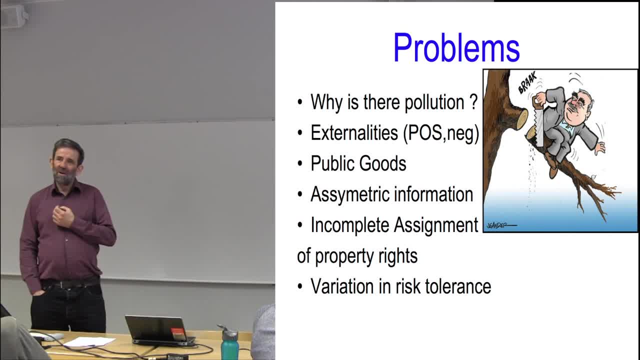 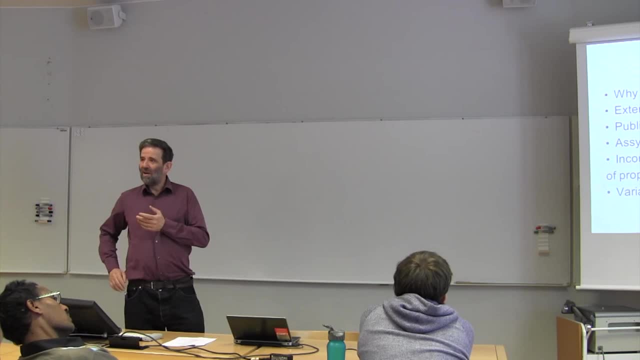 but the requirements for a market to work perfectly are draconian. We have to assume that all rights, that there are rights to everything, But we don't have. We have rights in Sweden, for instance, to land. typically Most land has an owner. 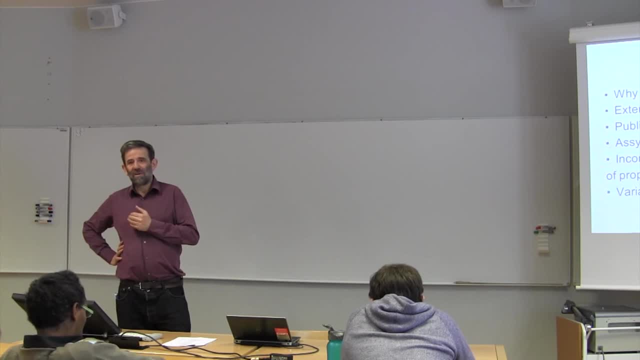 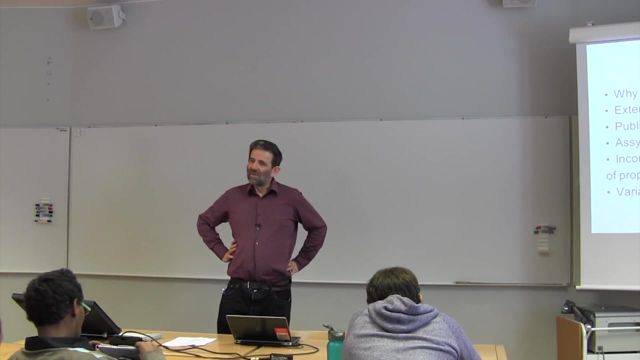 Not even. that is the case in all developing countries And in many places in Africa. there are land rights which are incomplete or insecure, But we certainly don't have rights to the atmosphere. We don't have rights to a lot of- There's a lot- of water. 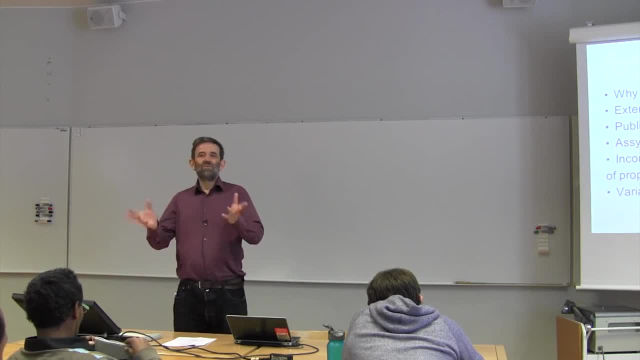 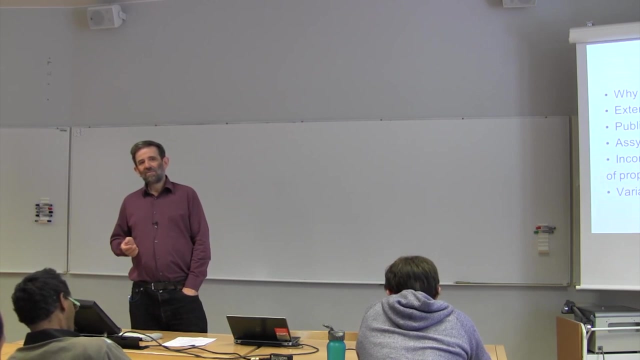 There's a lot of quite more subtle aspects. This room here is full of all kinds of radiation and properties. There could be, you know, contents of chemicals and so on. We don't have detailed rights on everything there. We make up rights basically. 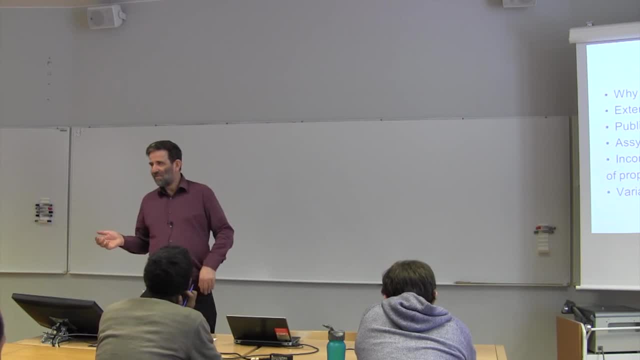 when we discover new problems. You go back to the 15th century. there were no property rights to radio waves. Today, of course, you can own a frequency like 98.9, something megahertz in some place. Someone owns that. 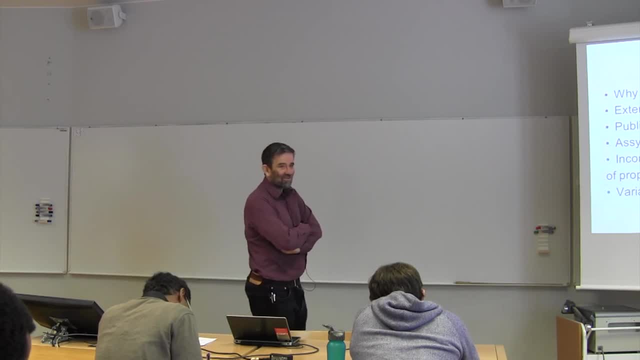 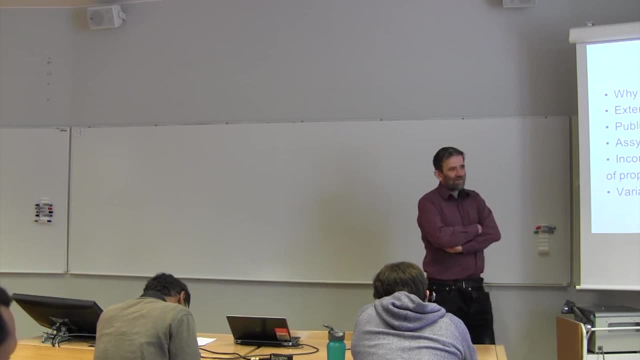 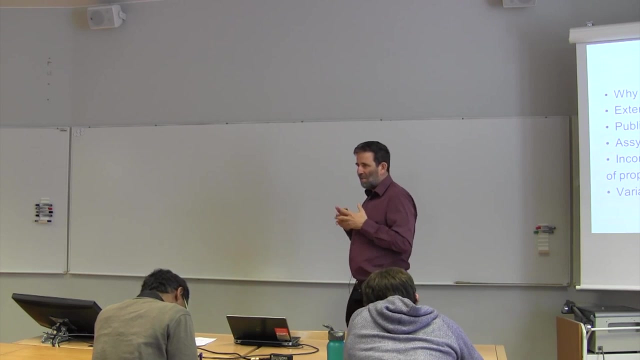 And you have to pay a lot of money if you want to use it, And you get into a lot of trouble if you use it without owning it. And so a market will work perfectly if there are property rights to everything and if those property rights don't overlap. 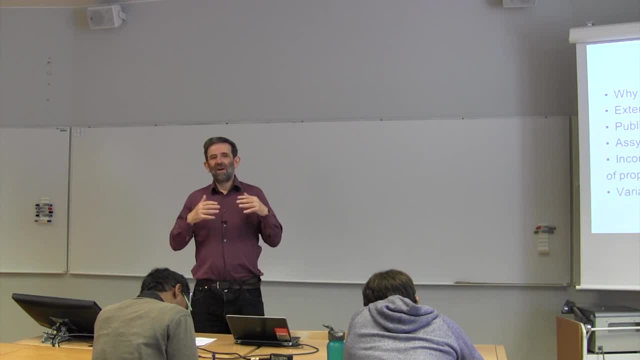 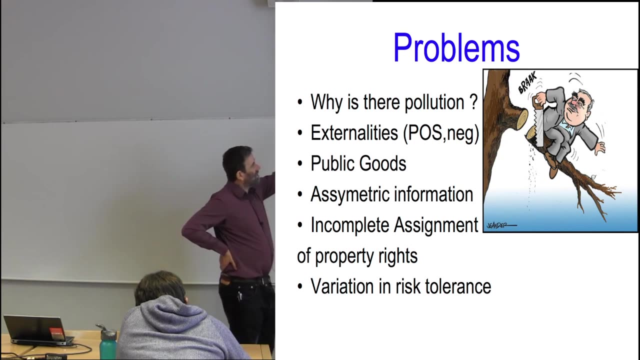 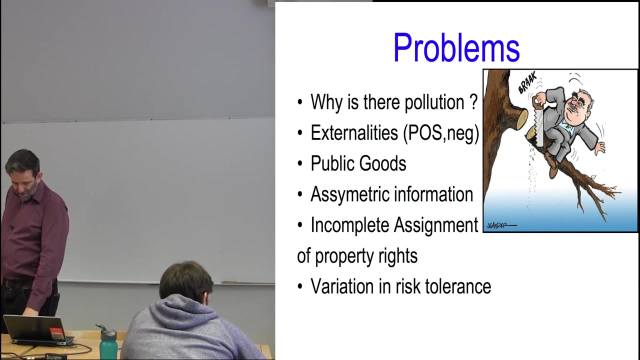 There's a problem if there are property rights, that kind of overlap, because then you get problems along the borders that are sort of related to what we are going to call externalities. Externality is a really fundamental and important concept. I have a 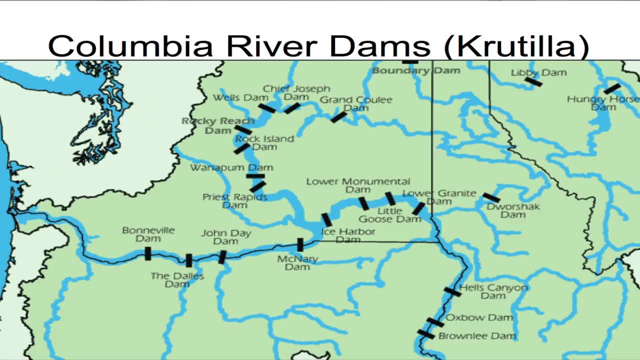 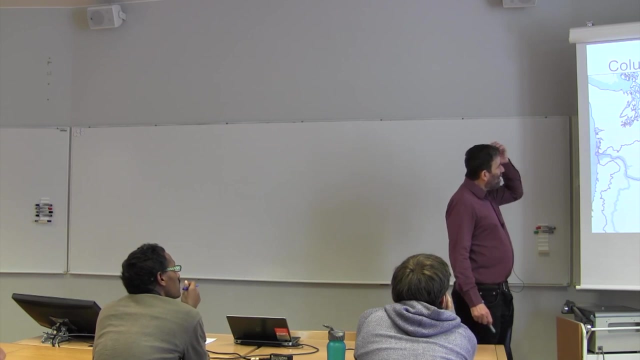 I have a picture here of the Columbia River. One of the first studies in environmental economics was written by a guy called Crutilla who got the first Volvo Environment Prize in around 1990.. And he wrote about the Columbia River And as anyone 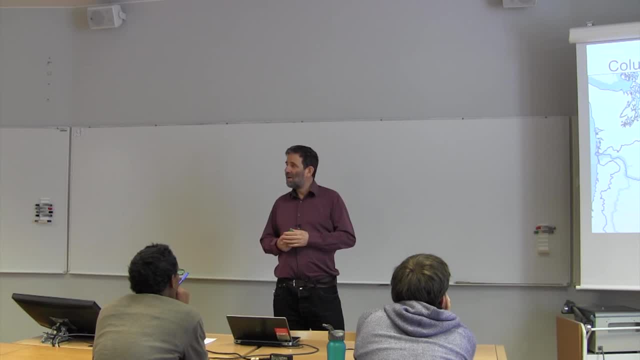 It's an unlikely question, I suppose, but does anyone of you know anything about dams? I mean, you could have a father who's been a hydro engineer, or someone, a relative, who owns a dam, or something. You know something about dams? 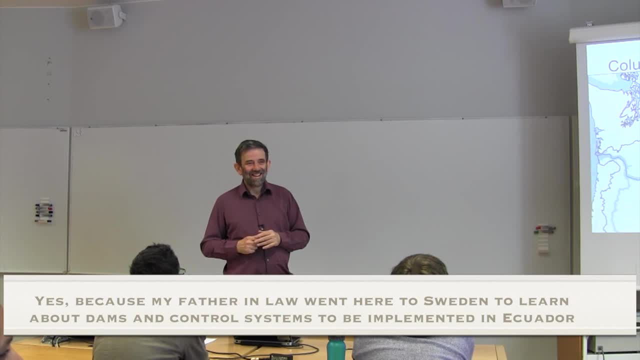 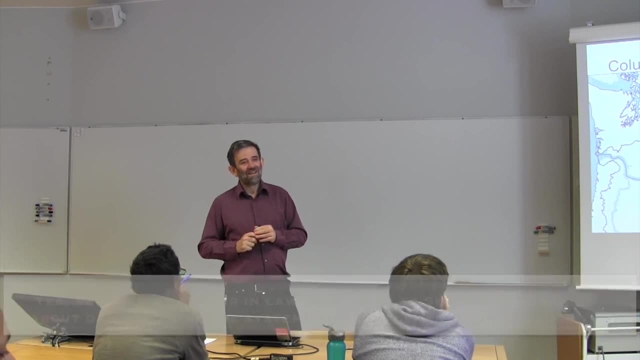 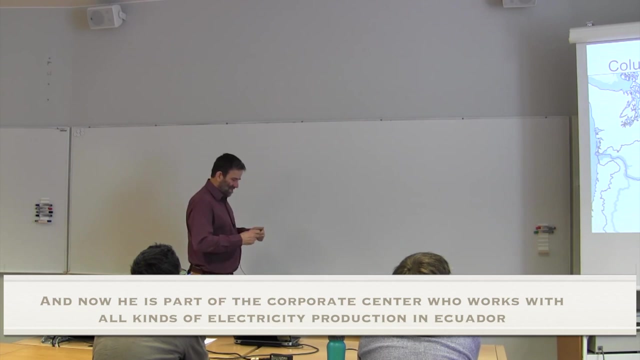 Yeah, That's great, But it's not all about dams, I mean. I mean it's not quite so fair. It's not just about dams. I mean if you look at soil corruption in the country and that's I mean. 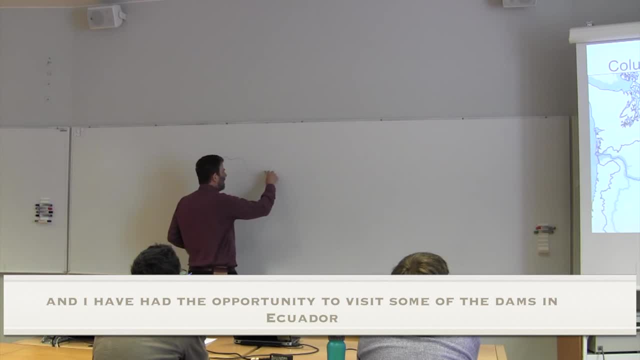 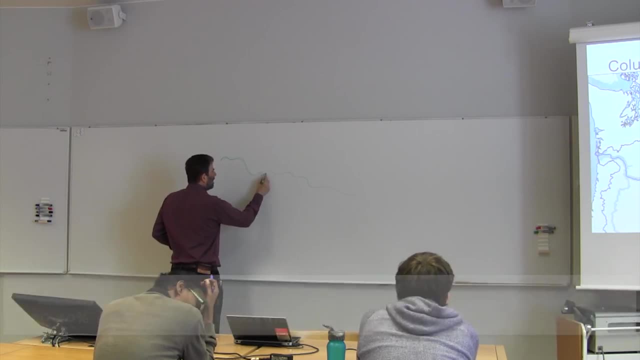 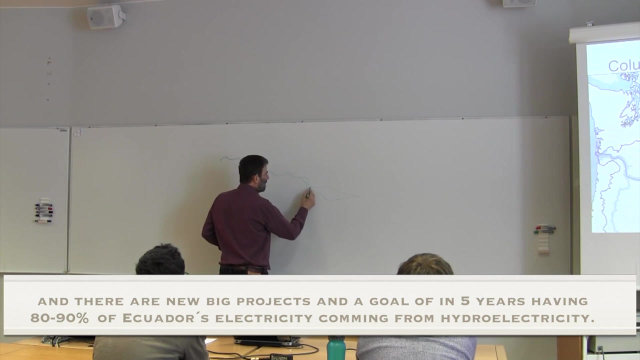 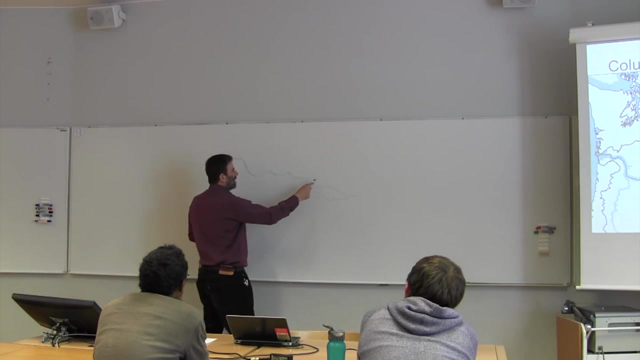 If you look at the See. so we have a river flowing this way and here we built a dam. and then we are thinking about building- or suppose we own a dam here as well. we'll make one more dam here, and then someone is thinking about building a dam here. 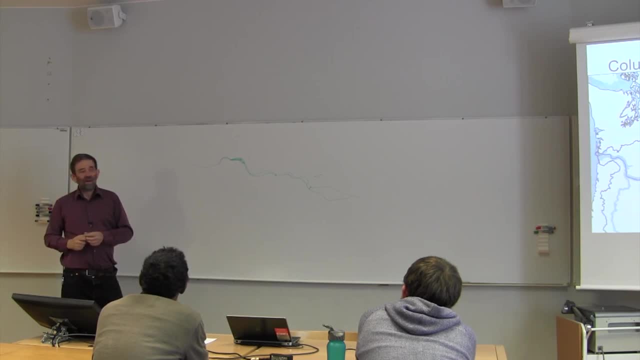 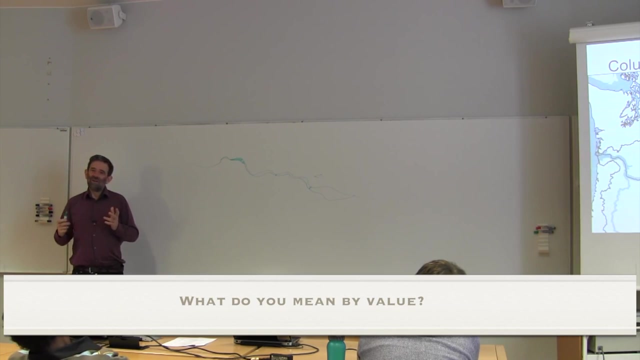 So there can be many dams on the river. And do you know what the value roughly? what is the value of a dam? How would you roughly know the value of a dam? Well, the economic value. Let's say it's for power. 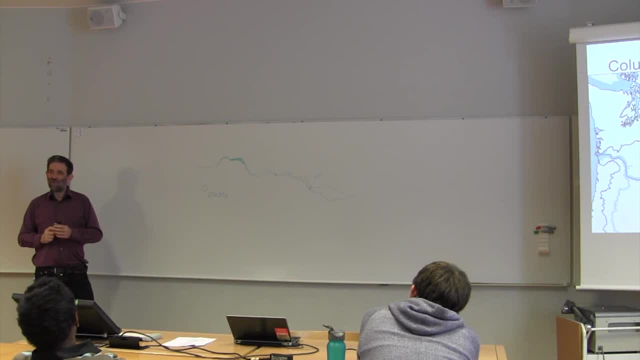 Then we have some engineers in the room. so how much power do you get from a dam? What are the two most important variables that will tell you how much height? Very good. And the other one, The volume of water. The volume of water, exactly. 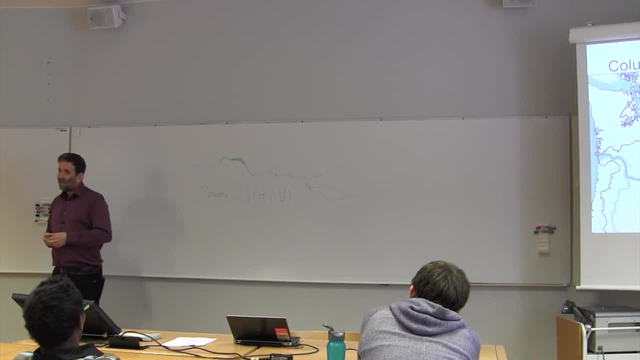 Okay, Now in many places, like in Sweden, there are mountains over here and it snows on the mountains all winter, and then there is a spring, a wonderful time when the snow sort of melts away and you get a rush of water. 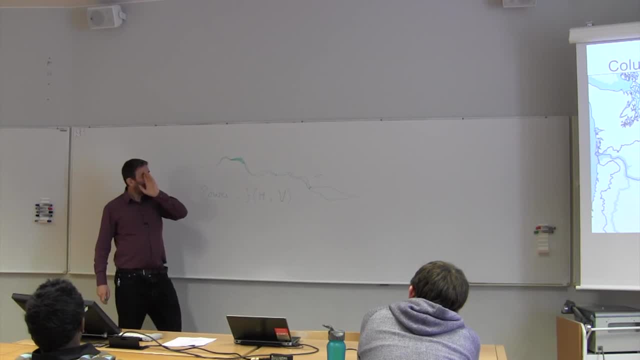 And what happens when there is a rush of water? All this water. first it fills up this dam, but there is so much water it does that in a few days And it flows on and it fills each dam, and then there is still too much water. and then 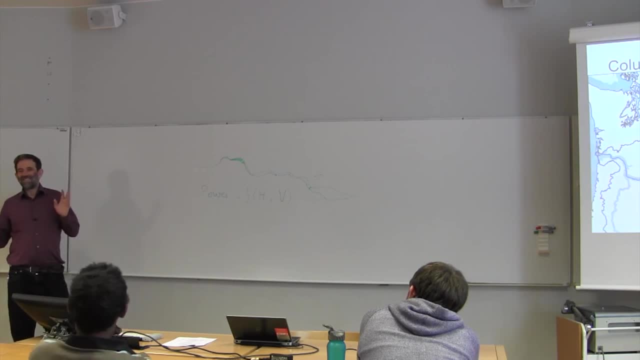 that water is, from the point of view of an engineer- is lost. I mean, of course, this is nice for the people who like watching the rush of water, but still it goes out to sea. So we own this dam here. 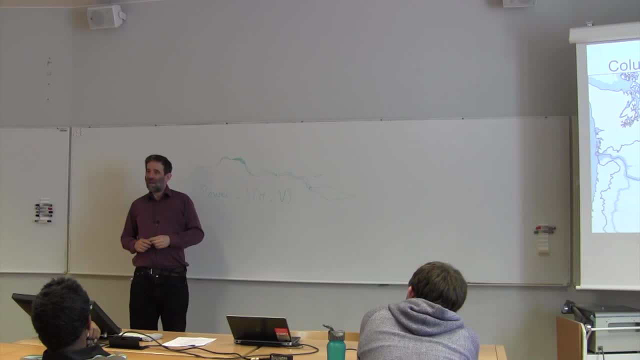 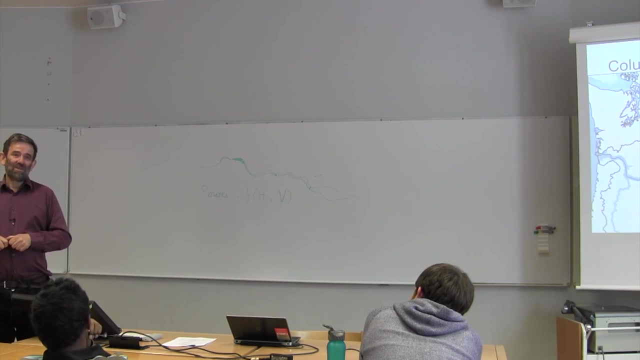 And we hear that someone is going to build a dam over there And they decide not to build it. What is our reaction? What do we say? Yoo-hoo? Well, we might say Yoo-hoo, But I'm actually going to claim, this time we're going to say the opposite, because suppose, 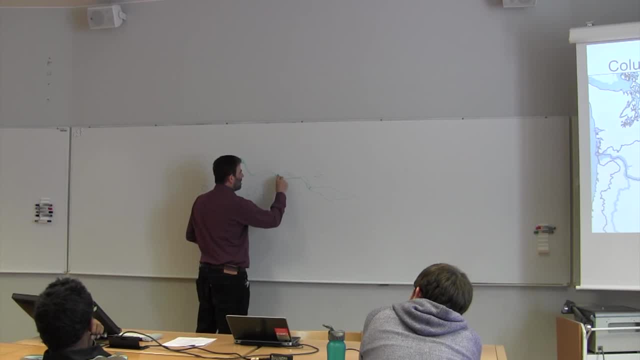 we do build a dam here, then next time there is a spring flood, the water fills up this dam, and then this dam, and then this dam, and then we start producing electricity. We start producing electricity here and then our water disappears as we produce. but these 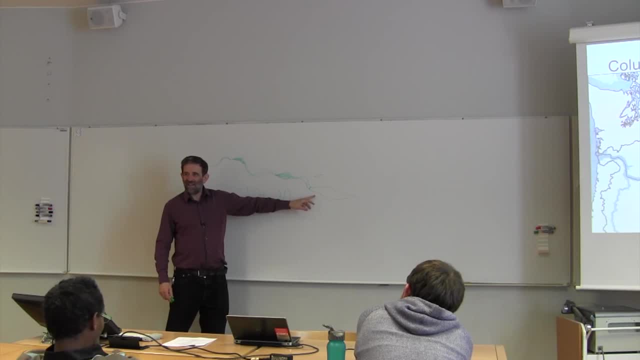 guys and these guys they are also producing electricity and when their water releases it flows into our dam. So they kind of built an extra dam for us And the value of my power plant here. this is V1, and this is V2, then it kind of it. 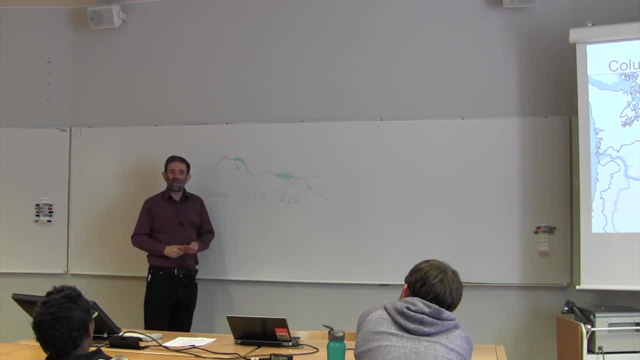 just went up. If they build a dam, my dam becomes twice as valuable. assuming the dams are equally big, I'll have twice as much water I can produce, not only like in July and August. I can produce July, August, September, October. 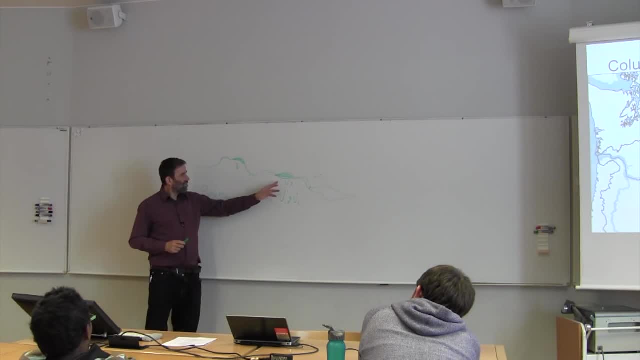 And so if they decide not to build, I might call them and say: hey, I have a lot of cemento, you could have it. I mean, their problem here is maybe they think it's not profitable. Well, if I paid the cement for them, maybe they will build it. 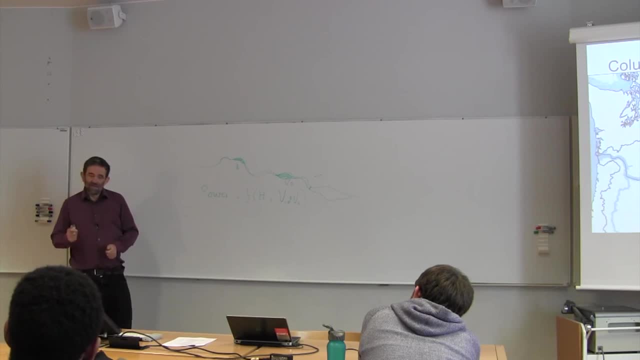 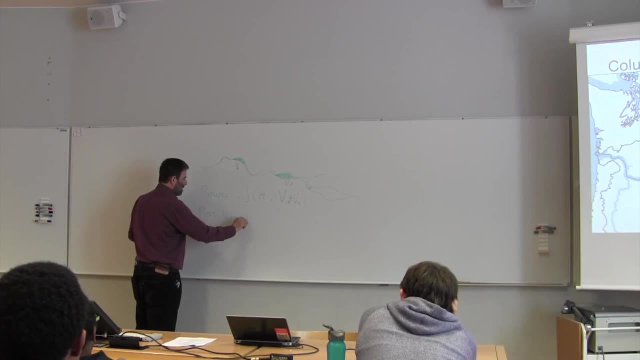 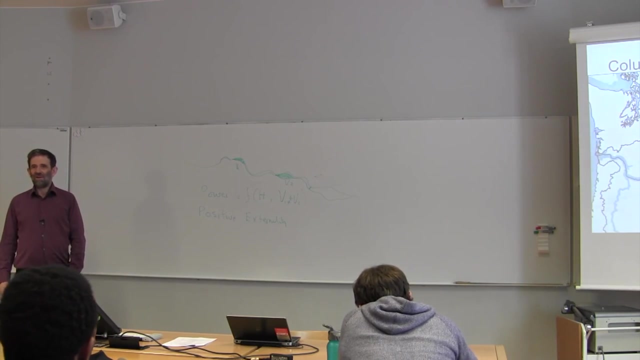 So what is this? This is a positive externality. It's something that affects my profit, but it's not in my control. It's in the control of someone else. We don't talk that often about positive externalities. We tend to talk about negative externalities a lot. 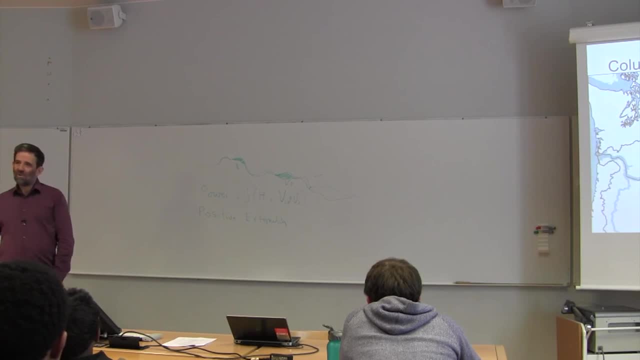 Negative externalities are the famous ones. I smoke and then you all get poisoned, or you know, or I make a lot of noise and then you can't sleep. A lot of environmental externalities are framed as disturbances. It's not in my control. 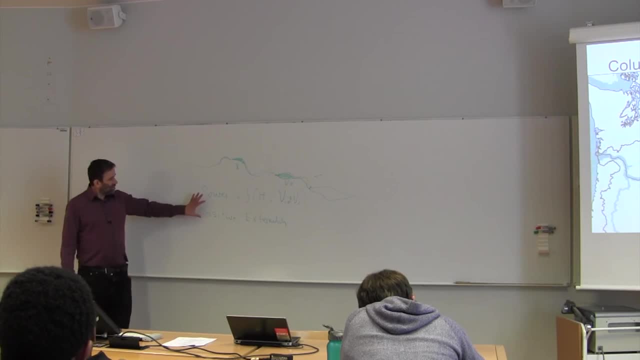 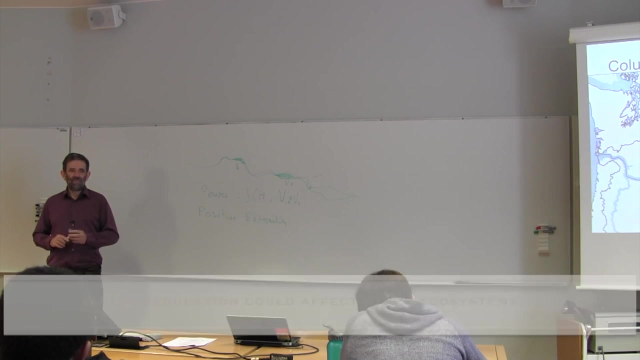 It's in the control of someone else. It's in the control of someone else. I think it's useful to think about the positive externalities as well. Of course, a dam has negative externalities as well. For instance, what are the negative externalities of a dam? 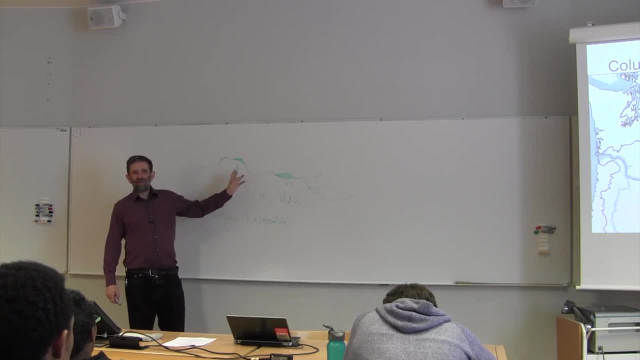 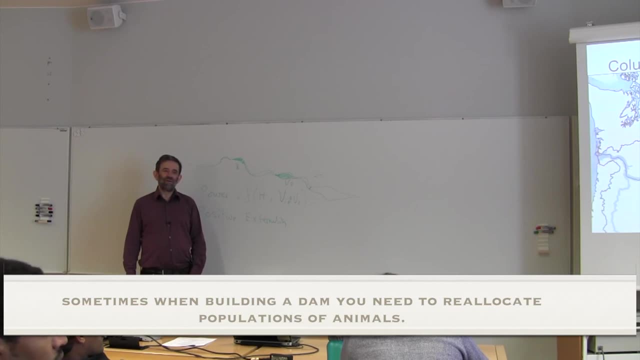 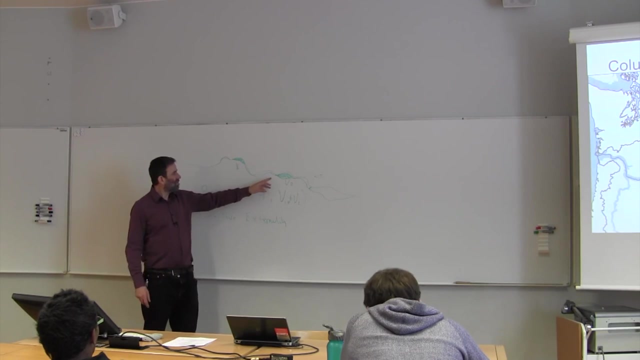 If there are some species of fish that migrate, they are in trouble, Like the salmon. Yes, they're usually in particularly tropical countries. someone will find a frog somewhere here that is maybe unique to that place, And so and there are sort of the endangered species acts, and so they have to try to relocate. 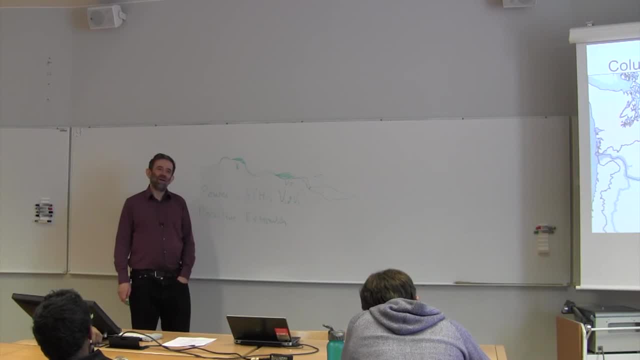 the frog or to do something, Ah, Ah. Of course sometimes there are some environmental activists who hope that if the frog is sufficiently important that they can stop the dam, So there could be all kinds of environmental effects. You cut down a lot of forest here. you change the ecosystem, you get a different composition. 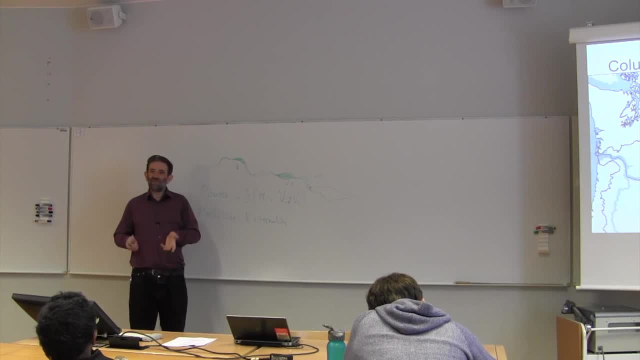 of fish You get. sometimes you get more fish, but you get another species of fish Sometimes you get. you get a lot of water standing still, So maybe you get an increase in malaria or dengue, or well, you get all kinds of changes. 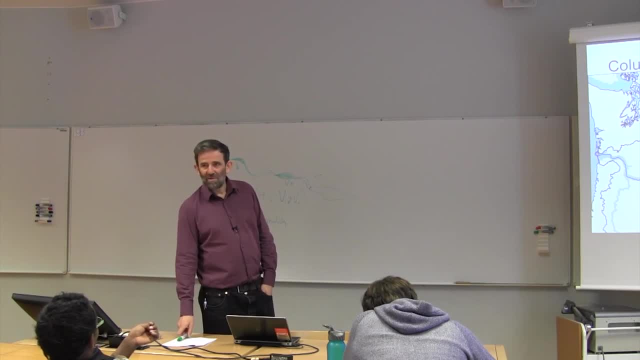 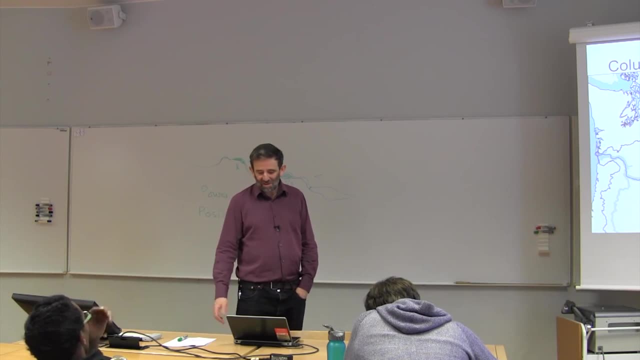 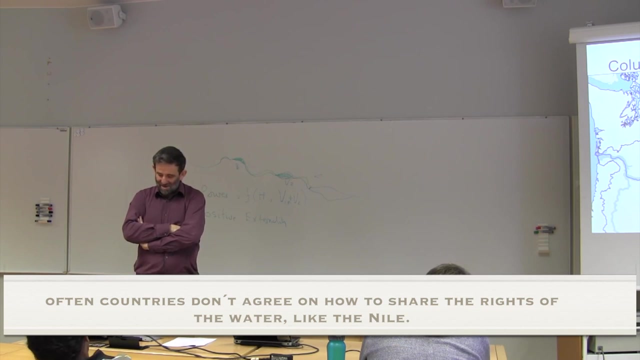 So there could be shipping. if it's a big river, shipping may be disturbed, or the other way around, It may become easier to do shipping. So there's lots of effects. Yeah, Yeah, Yeah, Yeah, Yeah, Yeah. And uh, why do you think that you know if, uh, someone takes the Nile's? 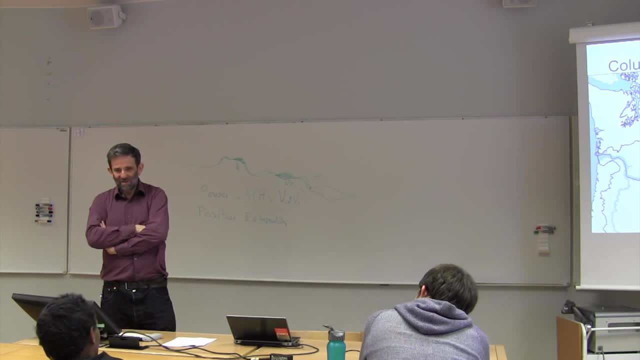 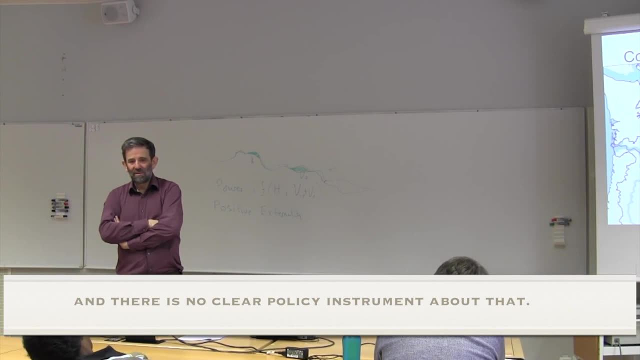 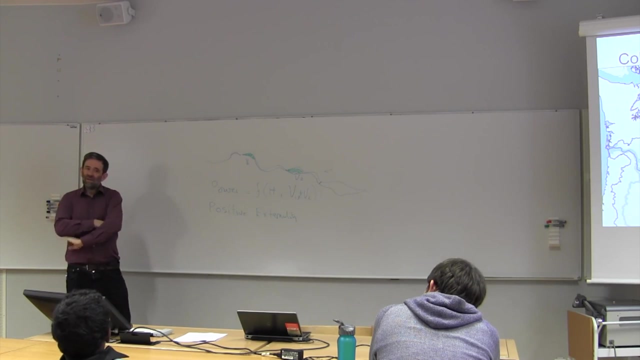 water, that Egypt would start quite a big war or do something. Yeah, I think that's um No, there's no, because there is not. it's not really clear who owns the right Does does Egypt have a right to an undisturbed Nile? 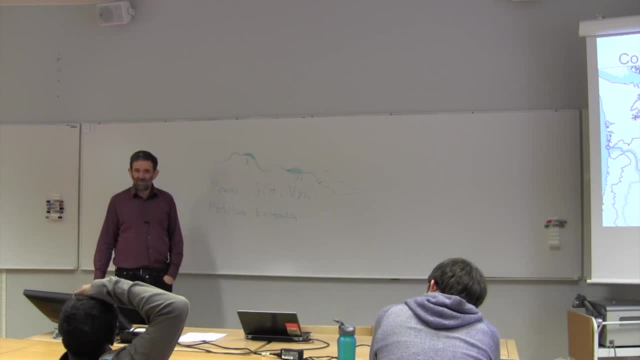 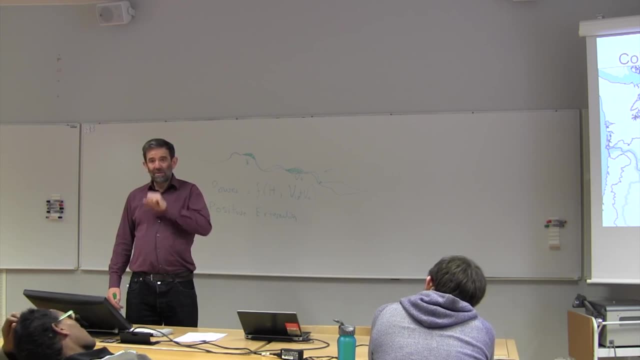 No, the Egyptian civilization has been there for thousands of years and those people live there because the Nile. I mean Egypt is heavily populated because of the Nile, there's no doubt about it. but on the other hand, the water rains in other countries, like Ethiopia, and so, if they feel, 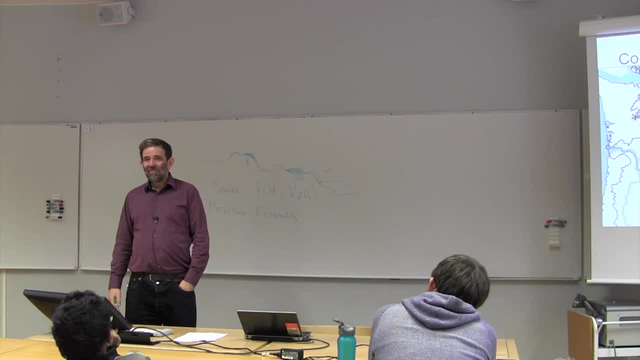 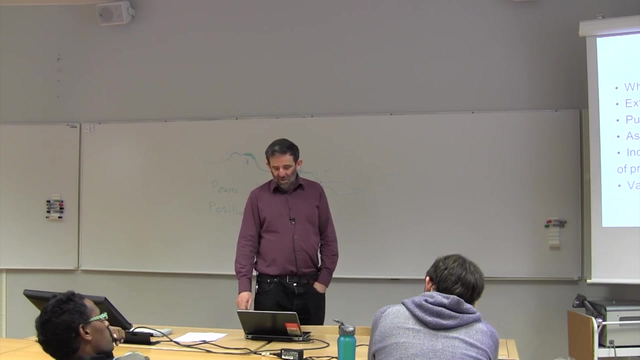 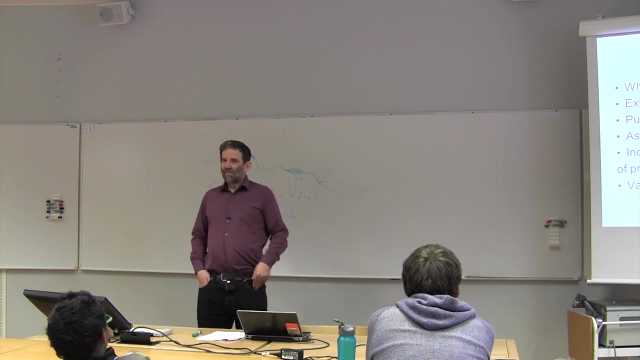 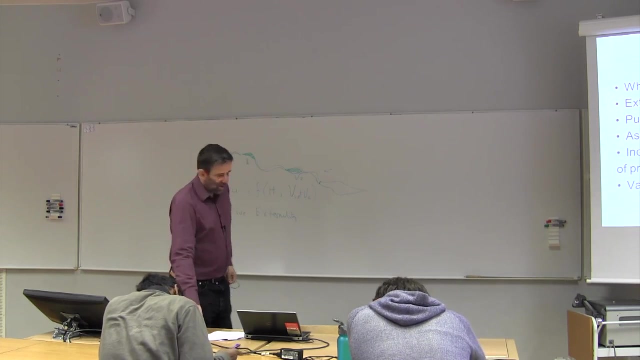 that, oh, it's our water because it's raining here, then yeah, there's a conflict of rights. that's not an easy conflict. so that is one area where we don't have property rights, and so there are externalities. if, if one person does something that can affect the property, the, the production function or the. 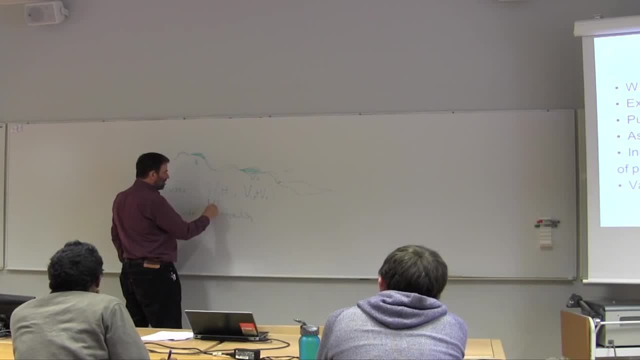 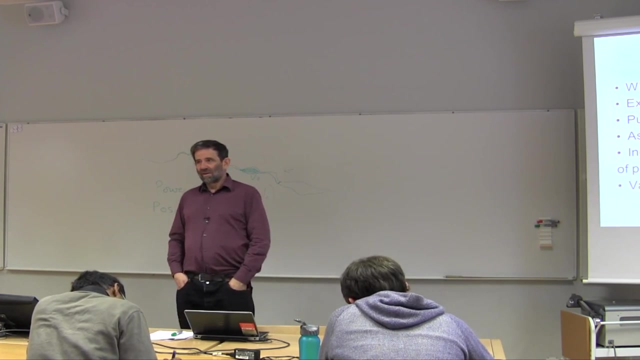 utility function, the utility function. but what we're looking for is this sort of kind of privilege of some other individual. so so when my profit function or what my utility function is decided by actions done by somebody else, not mediated through the market, then there's nothing very. 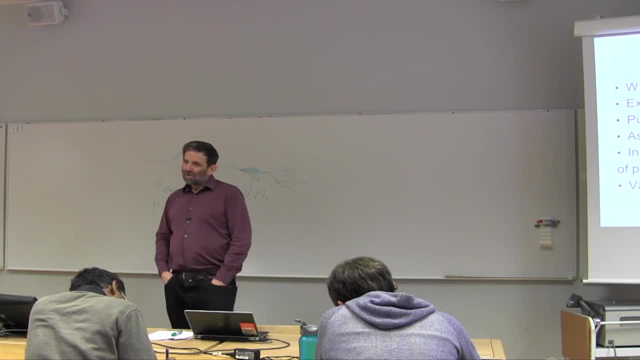 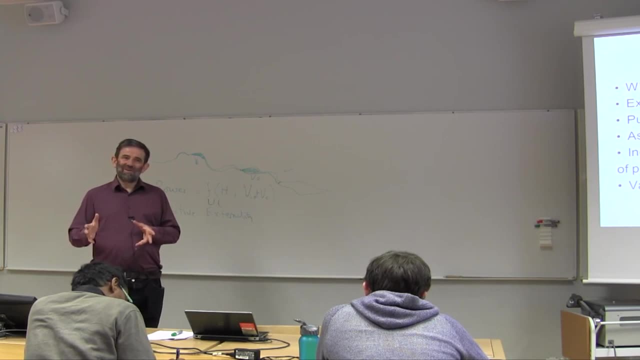 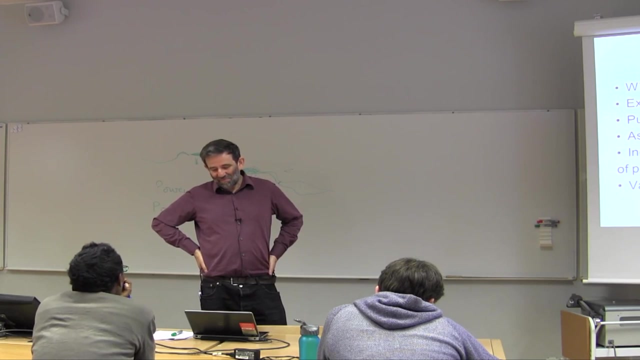 easily I can do about it except negotiate perhaps. positive externalities: it's often easier. you can offer to pay because there's actually some money on the table to share. negative externalities: you have a problem to share and there's it's somewhat more difficult. public goods are can be seen as a 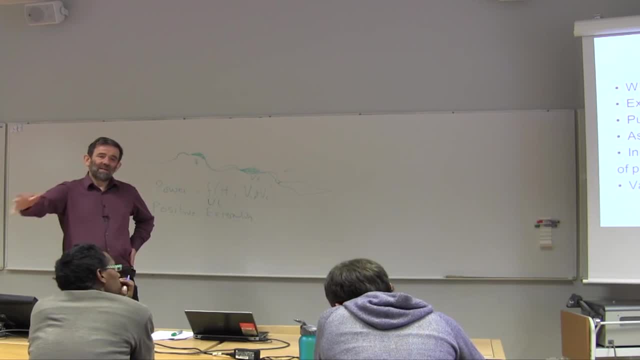 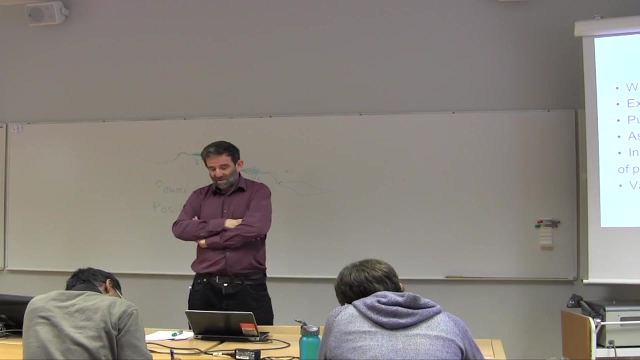 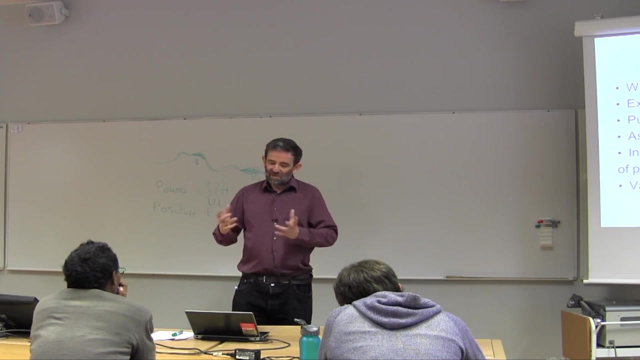 kind of externality, because it's it's an externality that one person has on everybody else, and so these are goods we consume together. they don't, they don't really fit into them. they can't be decentralized at the market mechanism. we can't let the market decide. we need politics to decide public goods. we need to both, we need to. 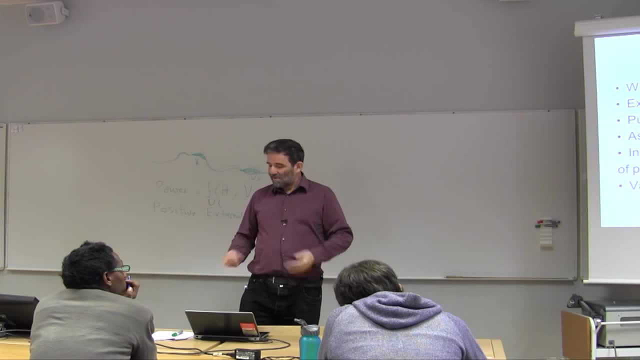 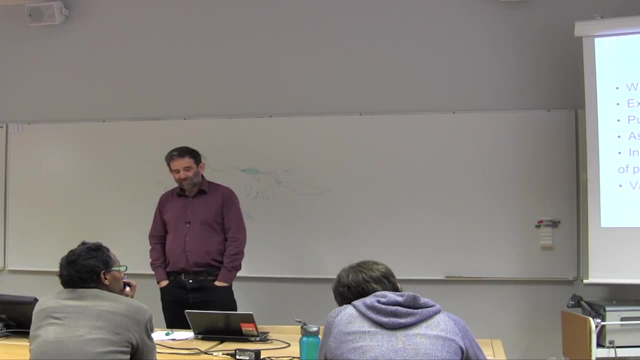 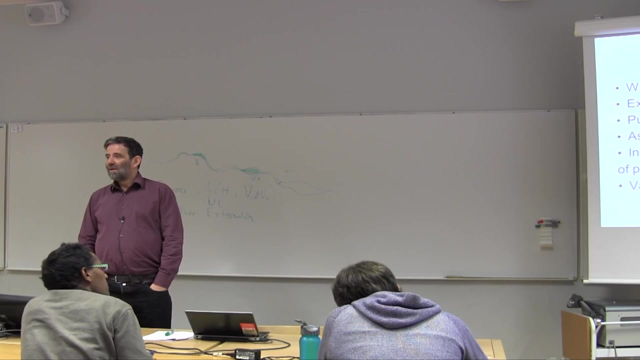 tax. we need to find other ways of allocating resources to public goods. asymmetric information is investment. the bottom line on our policy engagement is the health insuranceing process. important here. the market also assumes that we have, that everybody has the same, full, perfect information and that's typically not the case. very often the 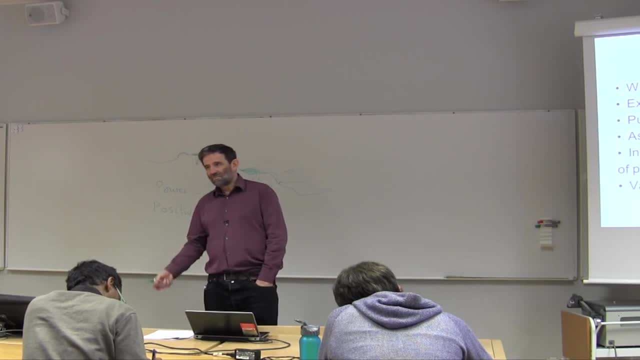 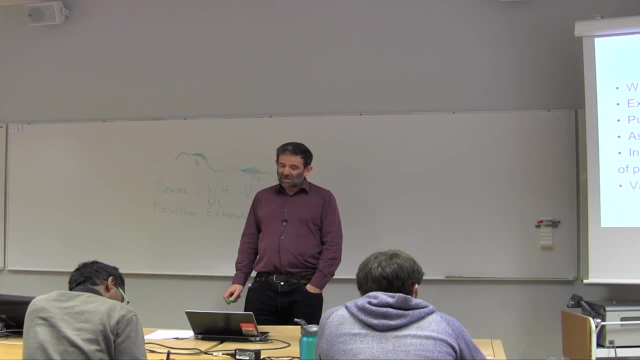 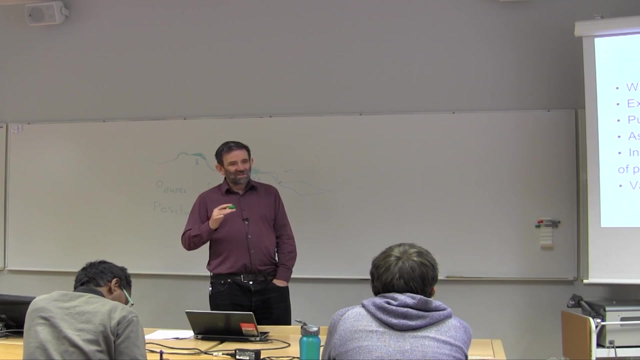 agents, like firms, know much more about their own production technology than other people do, than the regulator does. that's an important source of asymmetry. so if you're going to regulate them and you don't know their technology, you kind of have to guess what what their technology is, or you have to try some. 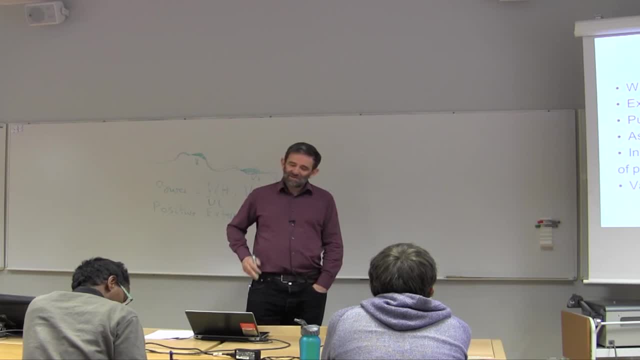 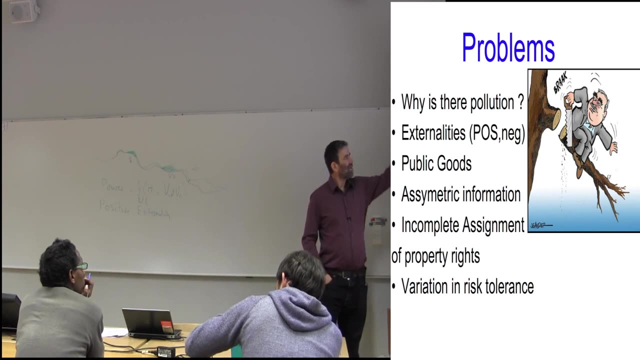 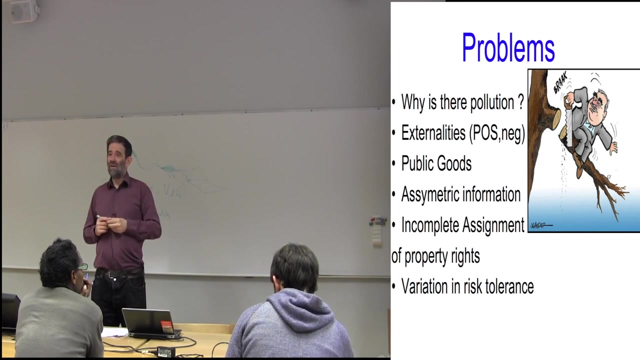 instruments and then see how they react and then it adapt the instrument. there could also be variations in risk with sort of a lot of this is sort of assuming that there that there is always a payoff, a payoff in dollars, X dollars, but sometimes there is not a payoff of X dollars. there is a probability. 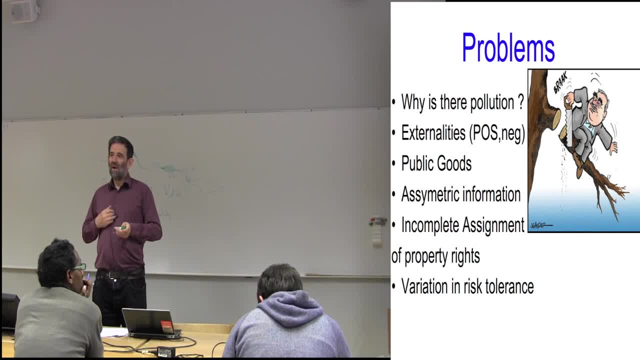 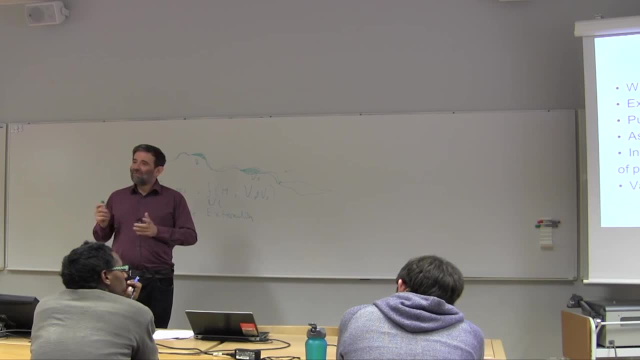 distribution of X and we may have different risk tolerance. a typical problem is the rich people, for instance, can afford to be more risk-loving. as long as the average return is high. it doesn't really matter to them if the variance is also high. so they can. they can take risky projects, and people with low incomes on the other, 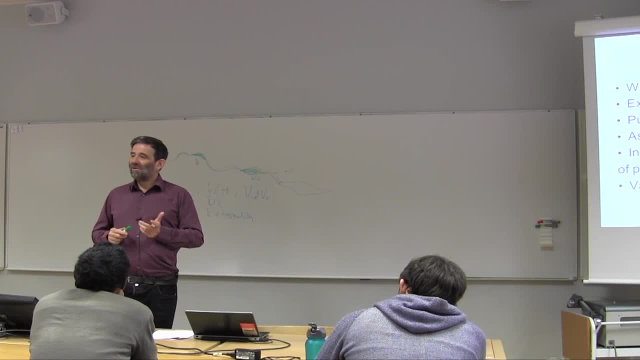 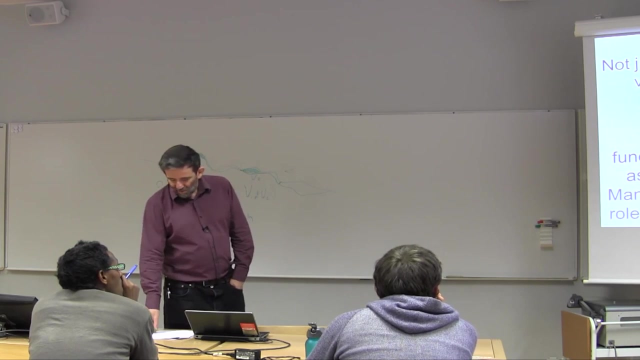 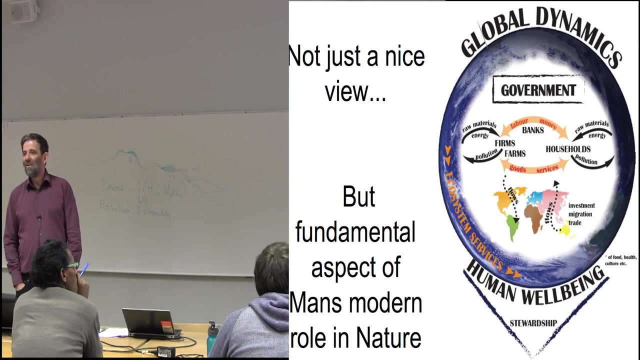 hand, they cannot afford to suffer too much risk, because if there is a year or even a month with a low payoff, that month they may in fact starve. now, the first examples of the classical examples of externalities that you find in in old literature were the, I think Adam Smith. 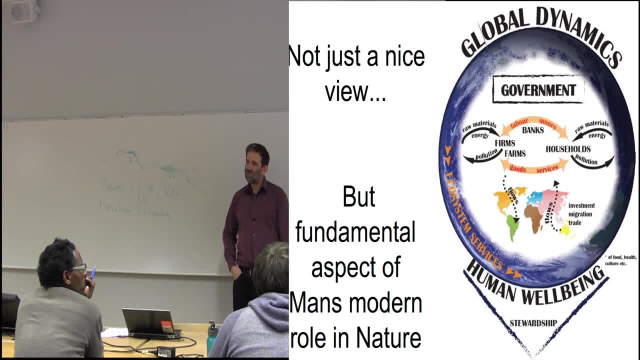 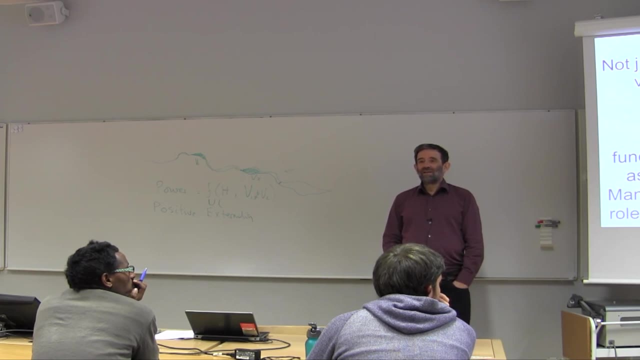 or someone- maybe Ricardo- wrote about how pleasant it was to walk by a neighbor's rose garden. that was beautiful. you sort of enjoyed the view and that seems like a pretty trivial example, like a relatively small problem. but we've come to realize that we are in fact facing really big problems, changing in, in, in. 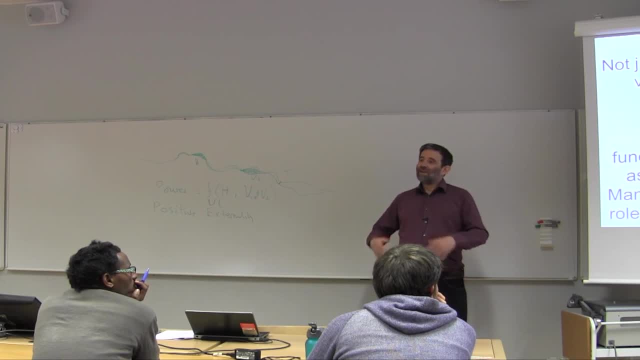 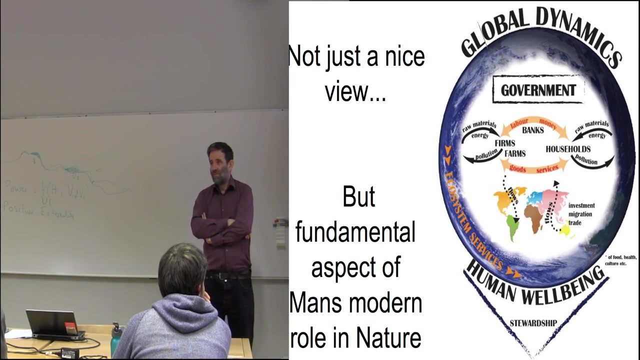 the ozone layer or changing the acidity of water, changing the composition of the climate or the atmosphere, that would change the time, but these things could threaten our life on earth and our well-being, our comfort. we used to study raw materials, natural resources, like one problem and then pollution like another, but in 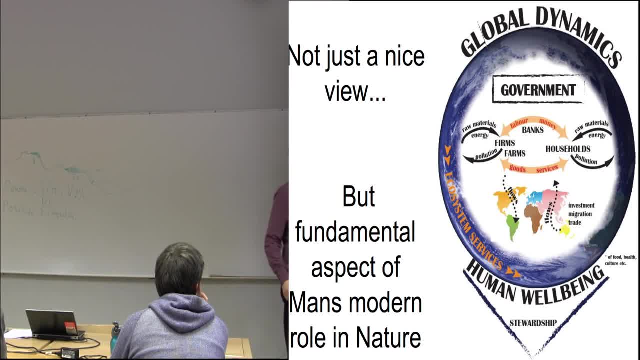 fact we have to understand now. there is a thin layer of earth where life is possible, where there is oxygen and water and photosynthesis, and it's the same place where we get our resources and where we dump our waste. in some sometimes, if you take a boat- take a boat to England, for instance. 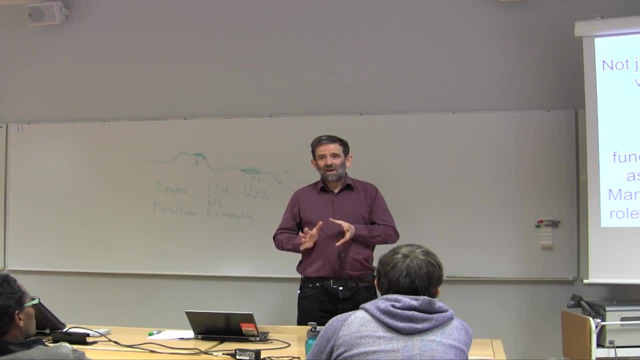 you know, across the North Sea it's very polluted, heavily used sea with as there's exploration for oil, there's shipping, there's all kinds of stuff and, yes, that's also where we get our food sometimes you look down in this water. you see, my goodness, is that where the fish in the like comes from? the weeds? 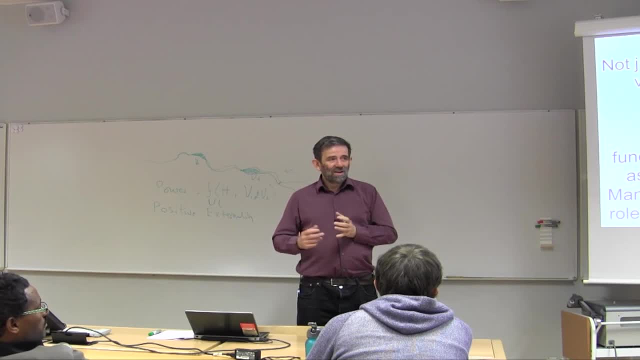 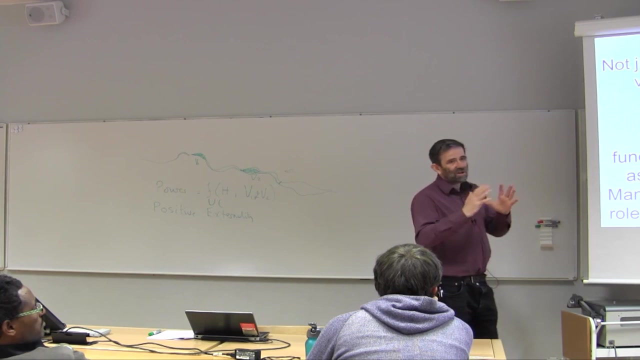 and yes, it is, and, symbolically, we are all like the people who live on the waste sites and scavenge waste, except that, of course, their plight is much worse than ours, but in some general sense we are all living in the same place. we're getting our food from the same biosphere, where we are. 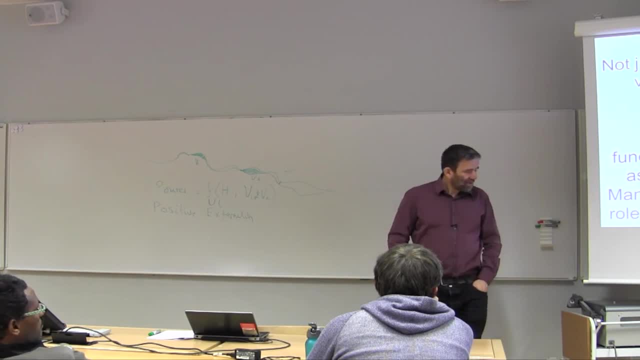 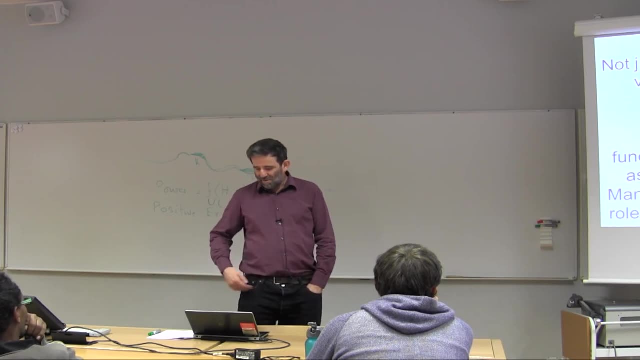 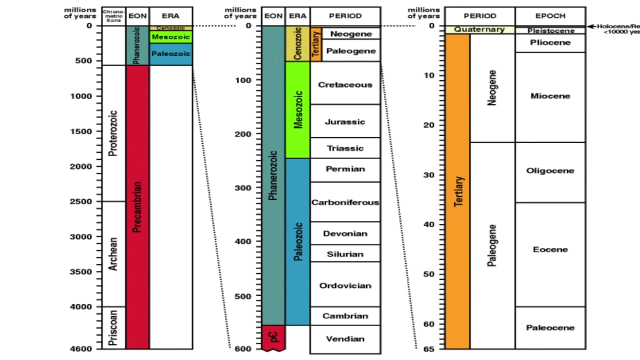 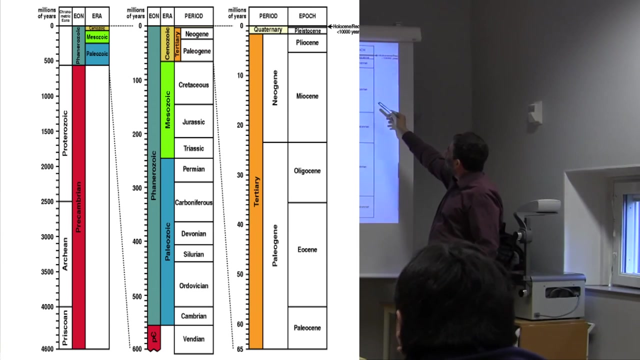 putting our wastes, And so it's a very big problem, big-scale problem. and have you heard of these ages that the what do they call geologists like to call the pliocene, miocene, eocene, paleocene? they all end up as the same. they sort of like to be like this: they go from one here to another and then they start to go from one there to the other. 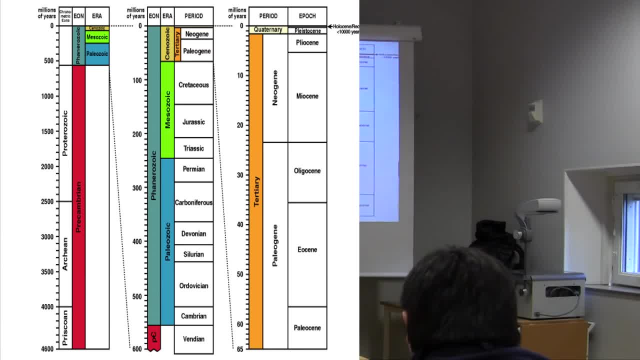 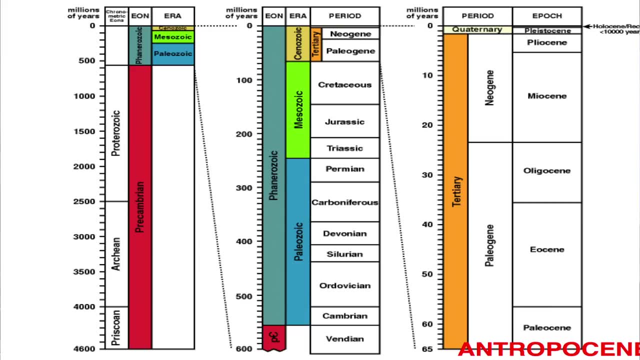 They all end up as the same. they sort of like to be like this. they start to go from one there to the other end with a scene. so that's now. someone very clever invented the Anthropocene. that is the geological age that we are now in, and by that we mean that this is. 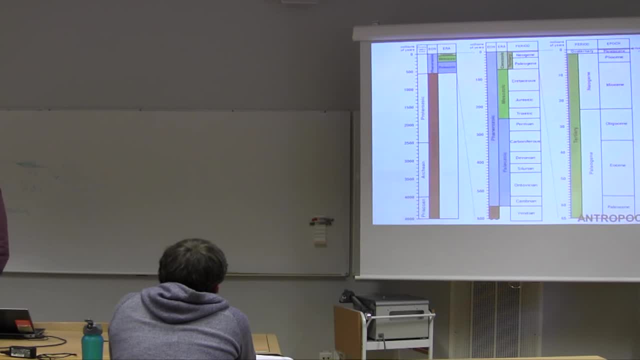 an age where everything on the planet basically is is determined by man. those of us who grow up in cities, we have this romantic view of the countryside. let's go out into pure nature and sort of see what pure nature looks like. well, there is no pure nature anymore. in fact there's one. one Swedish ecologist wrote: 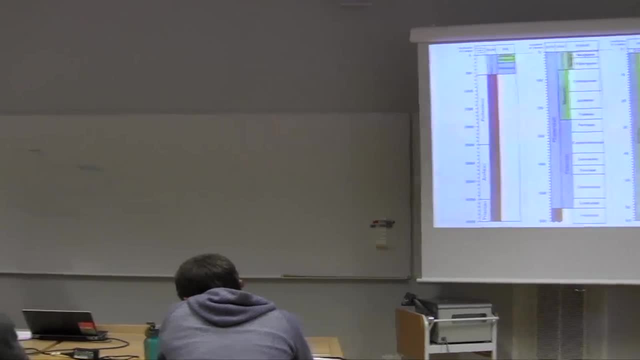 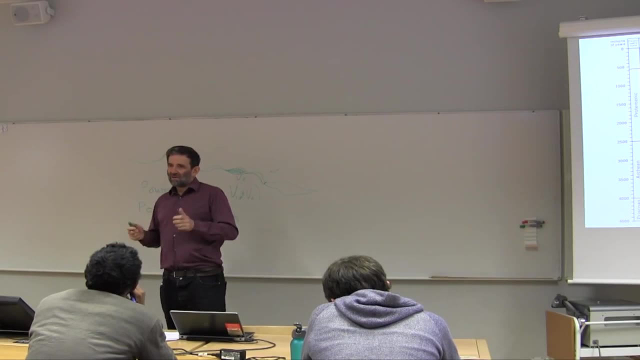 a sort of a history book of. he's an old man now and he wrote a history book of the environmental movement in Sweden and and he said that when he was young and started off as a young environmentalist. he said that when he was young and started off as a young environmentalist. 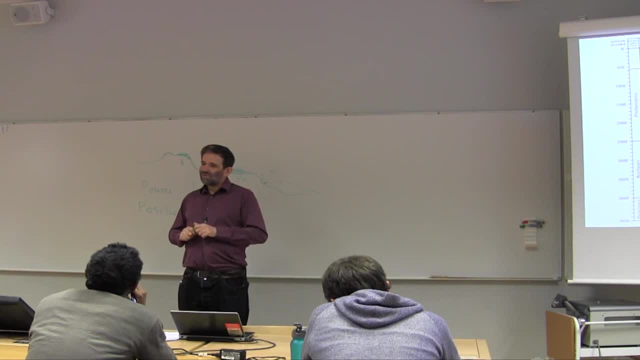 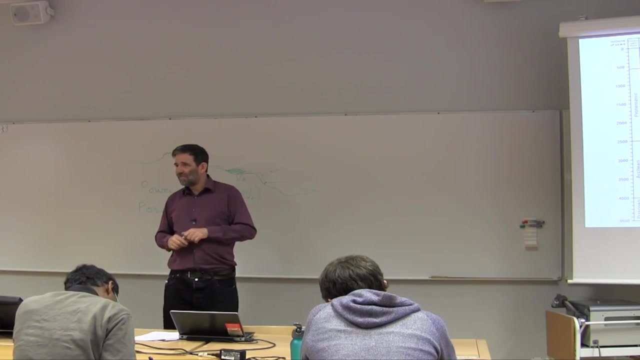 researcher. he said that we used to first we go to a factory. each factory had a little pipe and at the end of the pipe it would be terrible, it would be dangerous. we would go there, we would study, we would see that there was- basically there was hardly anything living there at all. and then we'll go 50. 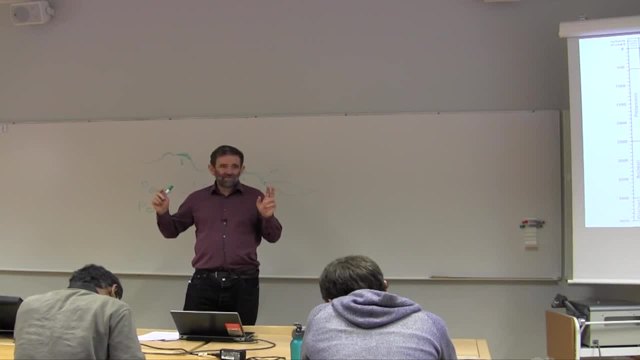 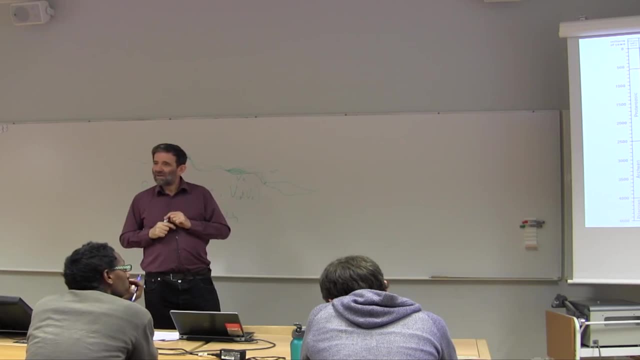 kilometers away, there'd be a place that was completely pristine and clean and we would study the gradient and see which animal survived, what concentration, and understand what the climate was and what the weather was, because we had to study the world a lot and of course we had a lot of changes, but I was not 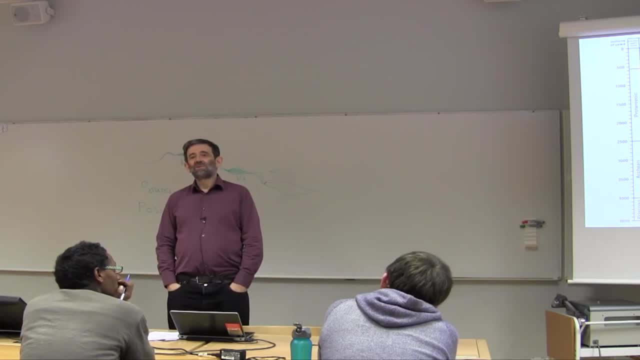 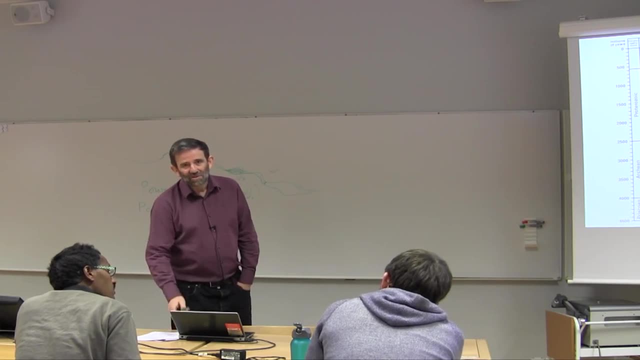 monitoring the climate of the world the last few years. in fact, I can't tell you how many changes we have made the. it's a lot of changes and I think I would say that the global warming is very, very important and the climate has changed as we live. we're living in a world with arid weather, which is very critical. 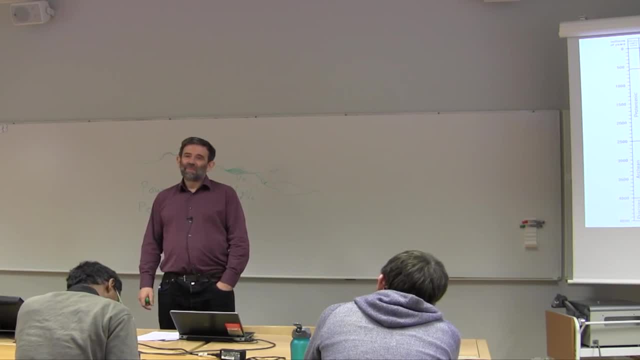 here in Sweden there's a lot of change. we're all moving to 60 degrees, so things are very different, and I think that's the most important. the way I look at it is that there is a kind of a global warming and that the climate is. 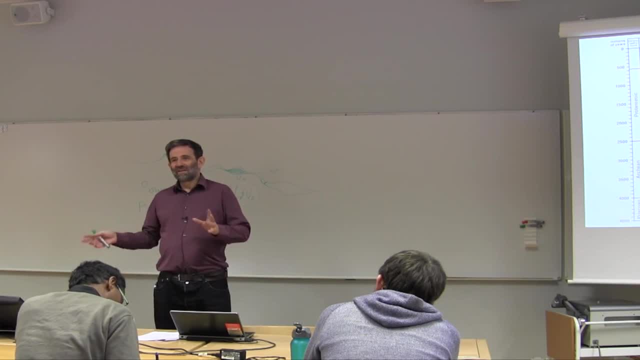 very different and I think that's the most important thing that we have to do in the world, for example, in the world of the climate change. and stuck to the right is no place that is really clean. so instead of short pipes, with all this effort, we now have much longer pipes. the OECD in the 1960s. they had a rule saying: 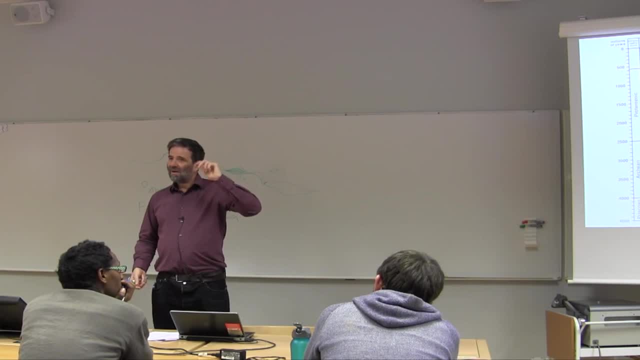 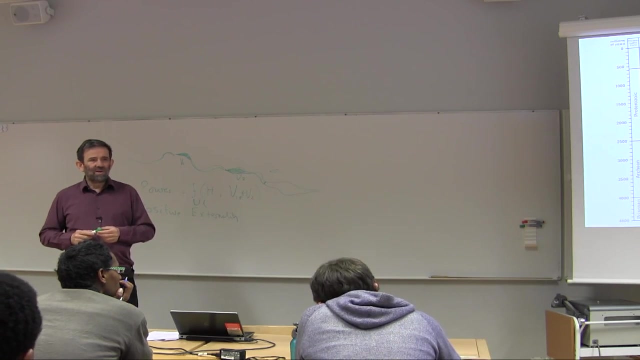 that you had to have her tall chimneys. that is a really laughable environmental policy. a tall chimney just means that you spread the pollution to a large area. it doesn't really mean that you are, is not? it cannot be called clean up right. you're not reducing the total amount of pollution and a lot of what we do is in. 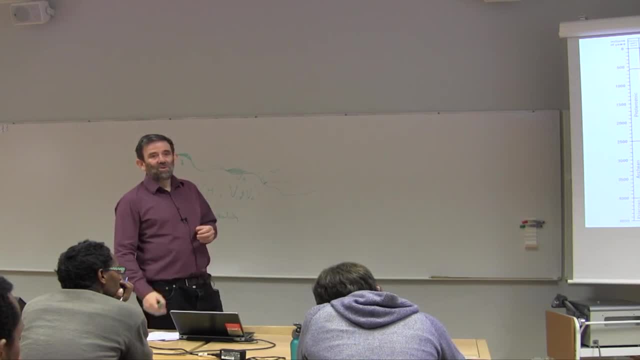 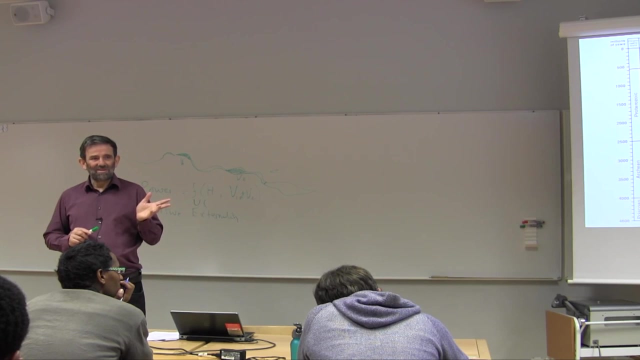 fact, moving the pollution further away. we call it clean up. even when we put a filter in a chimney, what do we do with the filter afterwards? and basically we throw it away in a waste dump and it rains on waste dumps, at least all Swedish waste dumps. it rains on them. so 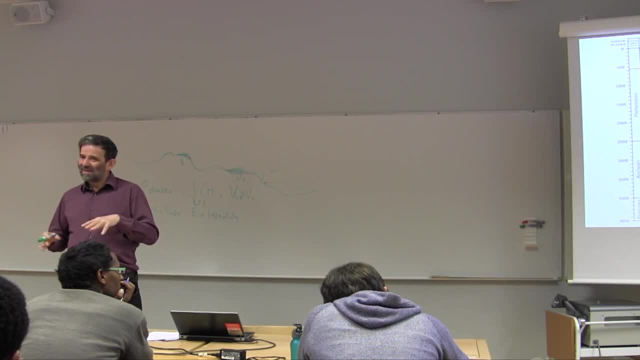 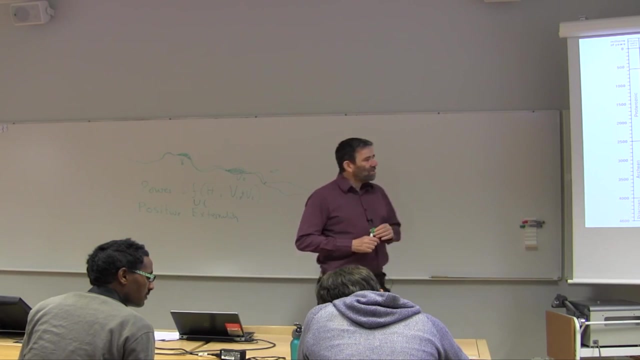 then the the content in the filter gets spread again. it gets spread somewhere else. now it is sometimes possible to do some real cleanup, but a lot of what we call clean up is really just moving the shit, if you'll excuse the expression, further away. so that means that all everything we are doing on this planet in fact is a is. 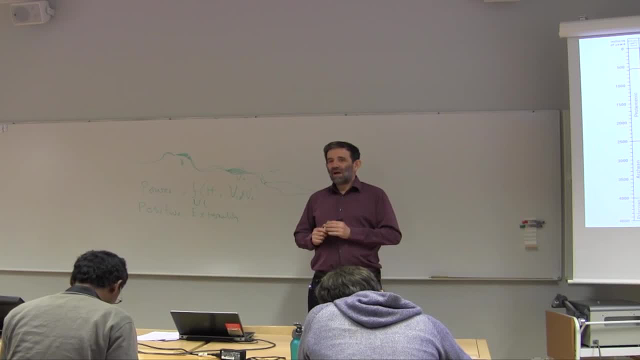 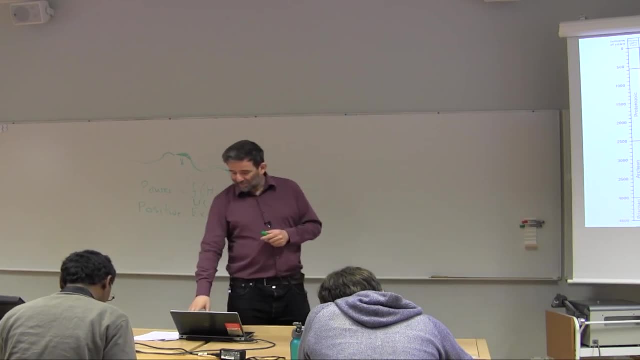 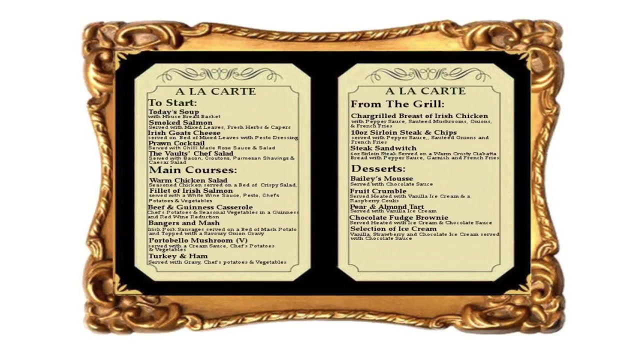 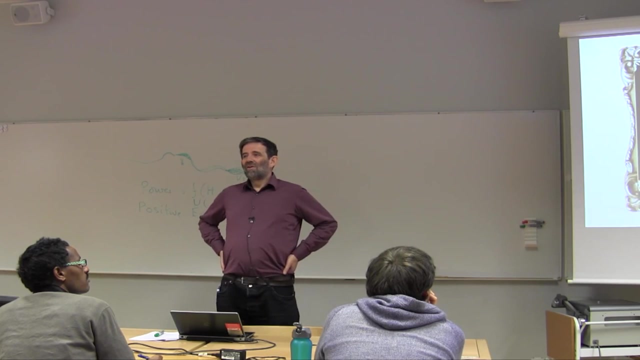 affected by us, and the faster we understand that and start managing it in a sensible way, the better. this is the menu for you will be for next hour. after we analyzed what, what, what the reasons for the problem are, we need to think of the, the menu of Of alternative policies, and I've been 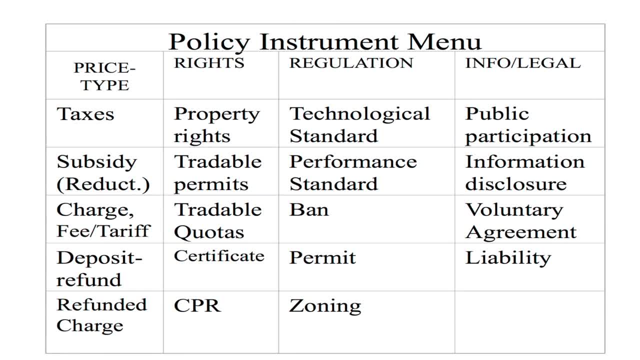 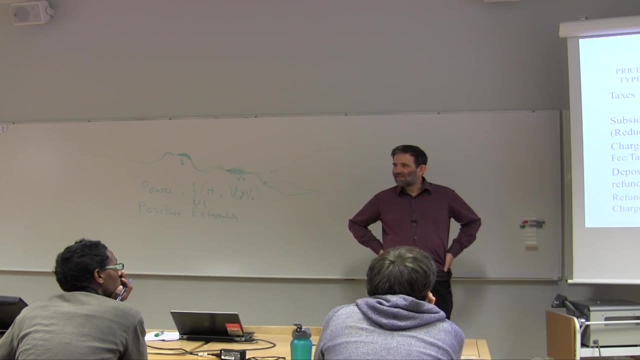 arlos working hard here to make a menu for you, and I've been working hard here to make a menu for you. different policy instruments that you could choose. I could just have this basically wants resistors and talk for many hours just about that. I will come back to this a few times.